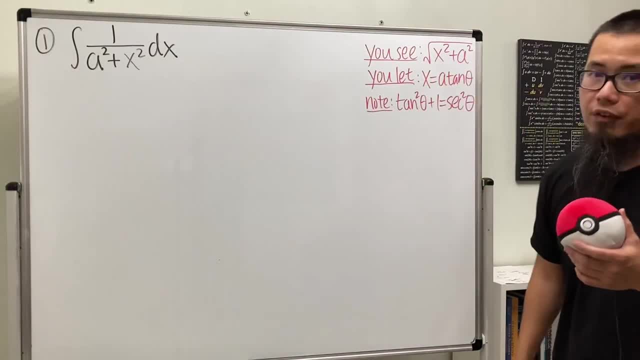 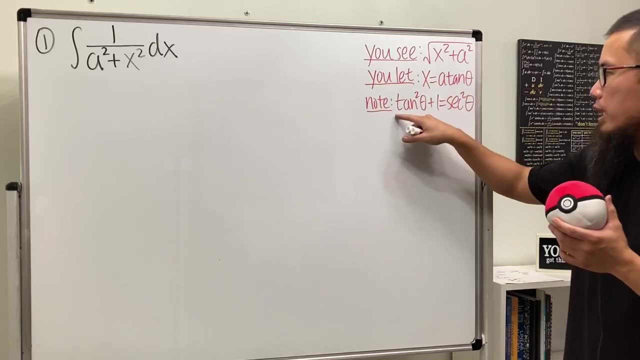 squared plus a squared, or maybe the other way around, because the order of the sum doesn't matter. And when we have that, go ahead and let x equal a times tangent theta, and you are going to expect to use tangent squared theta plus one is equal to secant squared theta. So now let's. 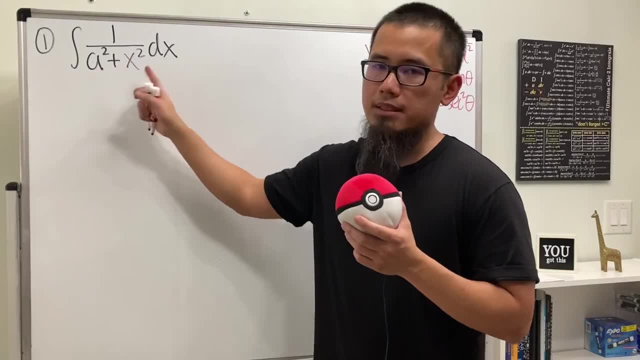 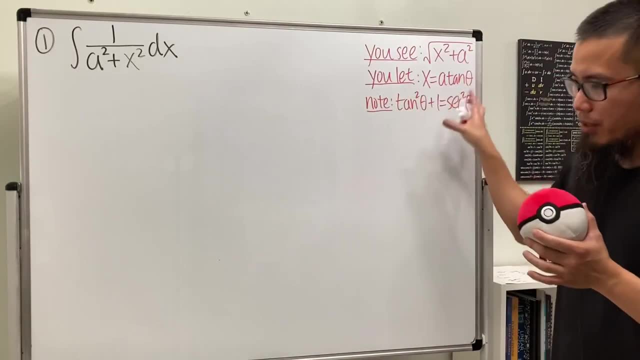 take a look at the first one. We have the integral of one over a squared plus x squared. There's no squared root, but it's okay. It's just that sometimes, when you have the squared root, this right here might be really really useful. but if you don't have squared roots, you can still use it. 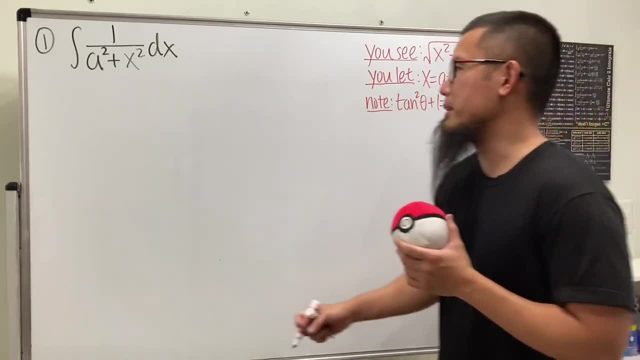 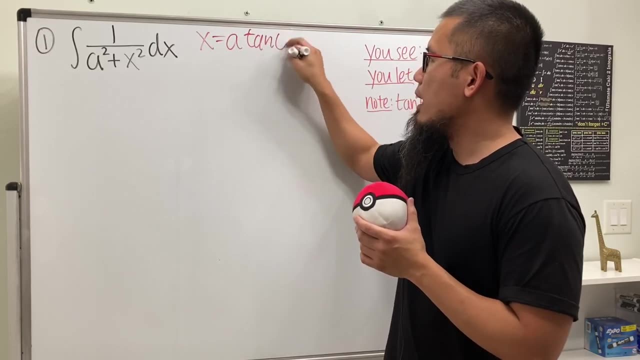 maybe right. So let's go ahead and proceed and see what happens Right here. let x equal a times tangent squared Tangent theta, and then we'll just do the usual business. So differentiate, we get dx equal a times the derivative of that which is secant squared theta, d theta. And now we can take this: 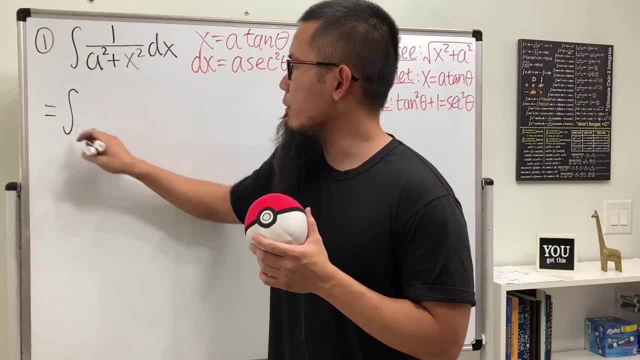 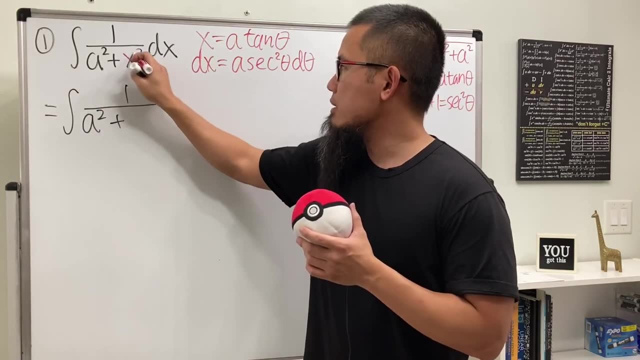 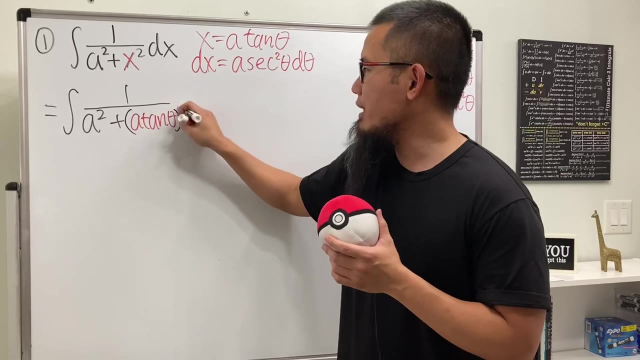 integral to the theta world. So here we have the integral, and we have one over a squared, plus here we have x, which is that Then the tangent theta with the a in front, and then we will just have the squared. 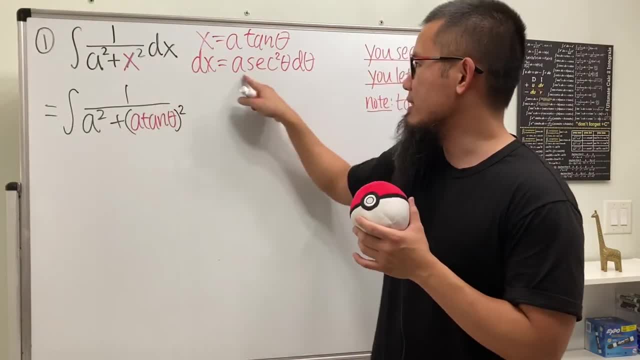 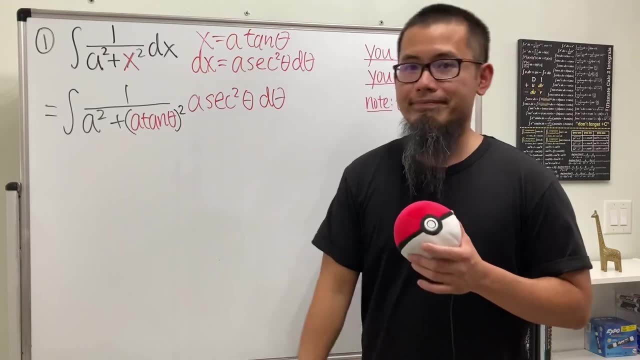 We are not done yet, because the dx is this, so go ahead and put that down A times. secant squared, theta d theta. Okay, now let's fix this part. Here we have a squared. Here we also have a. 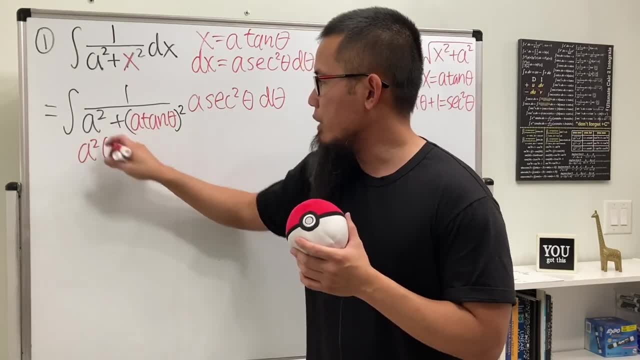 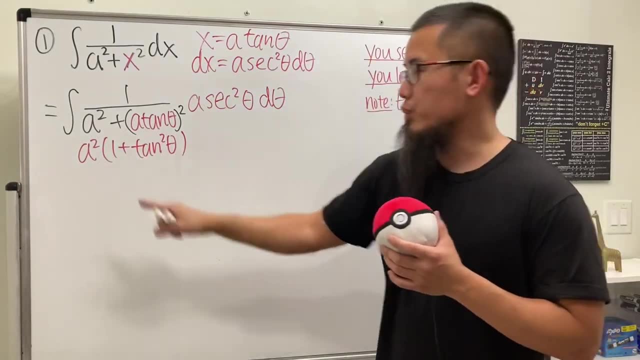 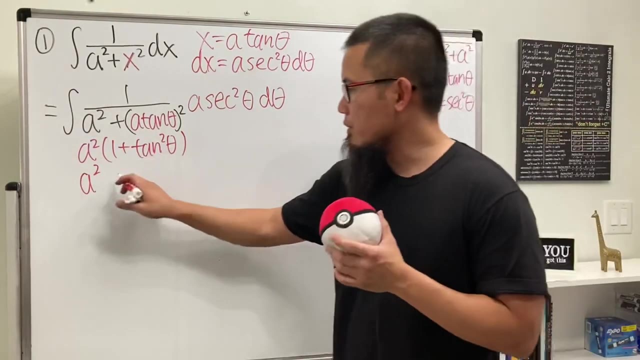 squared, so we can factor that out, Put that down here, and we are left with one plus tangent squared theta. This time there's no squared root. We'll just keep working on this. You see this right here. it's precisely secant squared theta, So let's write that down. And now here's the DO, As we can see, 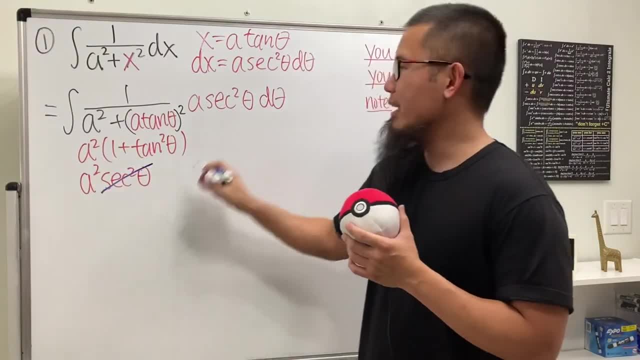 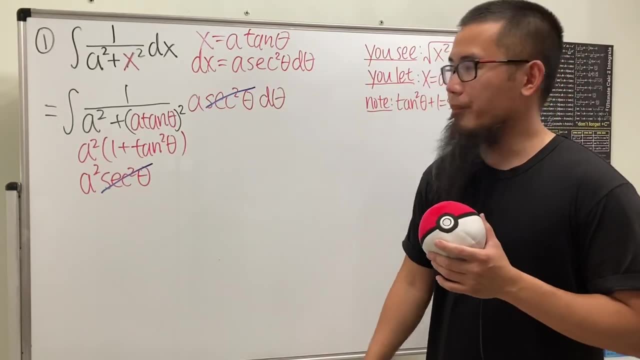 right here. we have the secant squared theta on the bottom, and we also have the secant squared theta right here, so they can cancel out completely. But be really careful, though: This is only a to the first power, but this is a squared on the bottom, So we can only cancel one of them out. 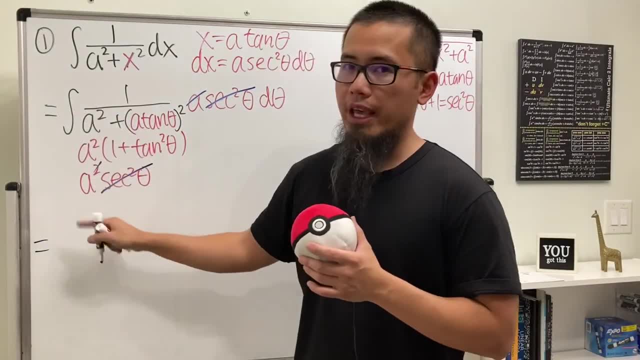 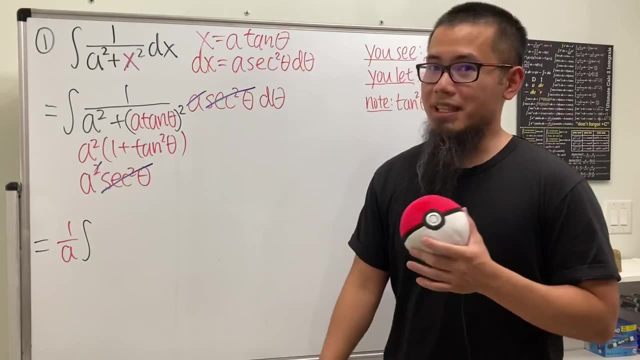 So this right here will give us one over a squared. Okay, let's just put that all the way in front of the integral, and then we have the integral And the rest of the things cancel out already. so we just have one in the theta world. 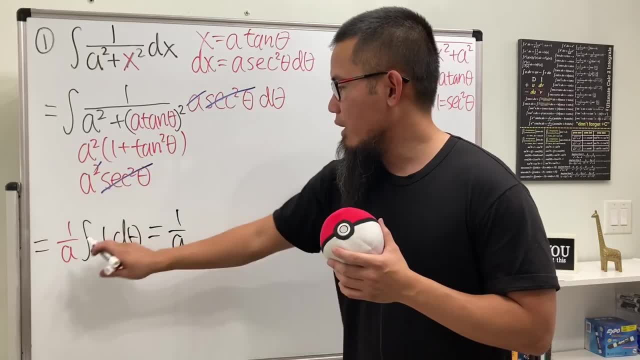 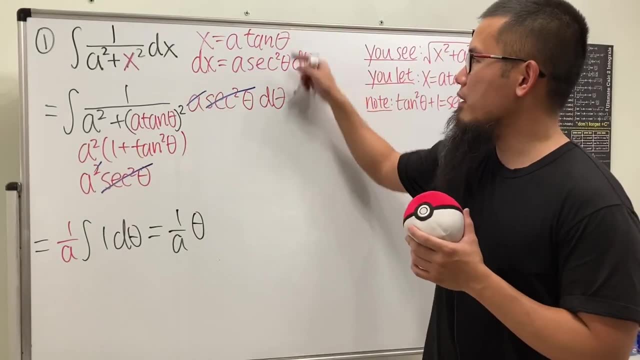 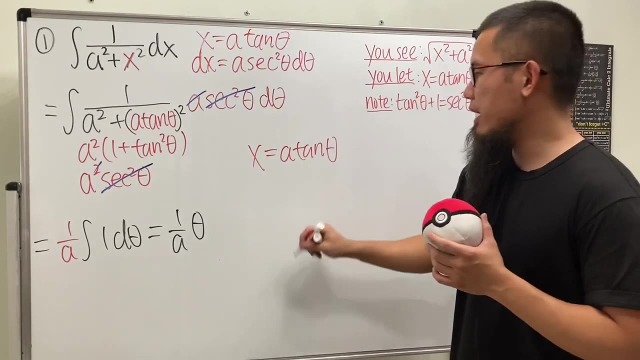 So this right here is gonna give us one over a. the integral of one in the theta world is theta. So now to figure out theta, we'll just go back here. We know x is equal to a times tangent theta. Divide both sides by a, so we are looking at tangent theta. that's equal to x over a. 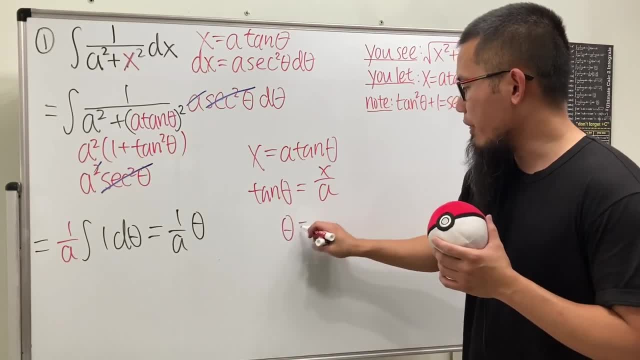 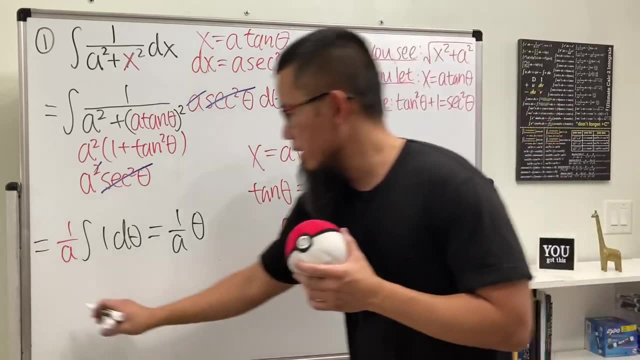 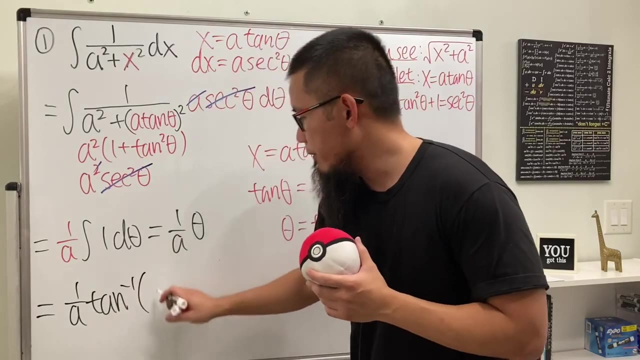 To get theta by itself, we just do the inverse on both sides. so theta is equal to inverse tangent of x over a. So we just put this right there. So finally, ladies and gentlemen, we will have 1 over a times inverse tangent of x over a for our answer. 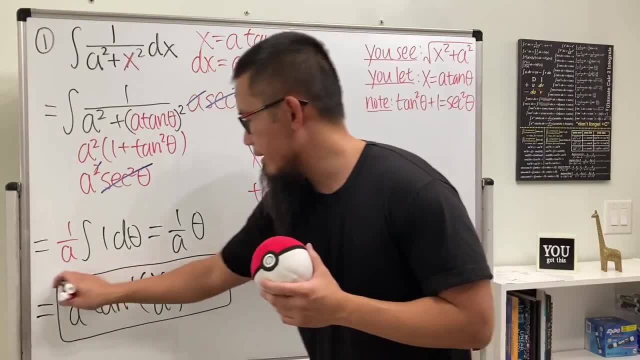 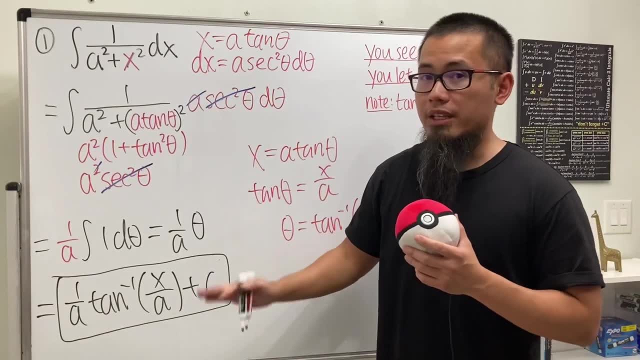 And, of course, put on a plus c. This, right here is it, And this is the standard result. You are going to remember this result right here, so that later on, when you encounter this, especially when we do partial fractions with rational functions, integrals. 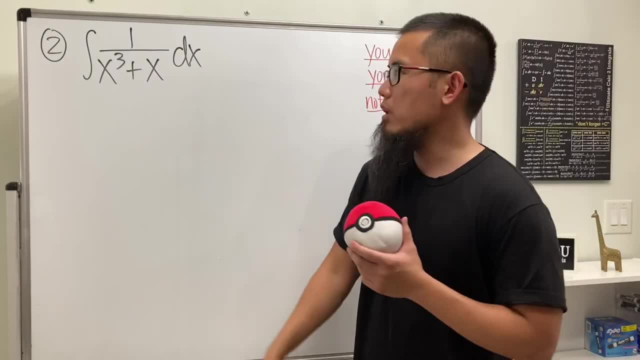 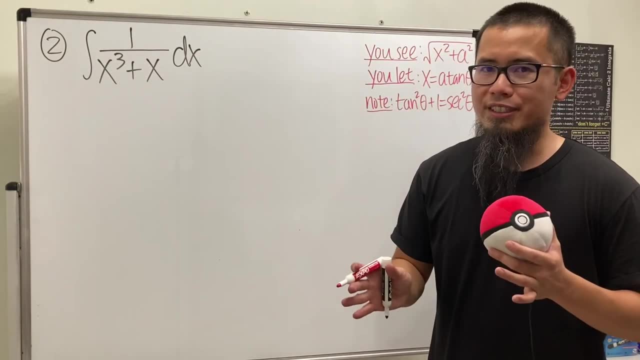 we'll be using this quite often. Okay, for number 2, we have the integral of 1 over x plus third power plus x, And you don't necessarily have to do tricks up for this. but since we are doing the tricks up, 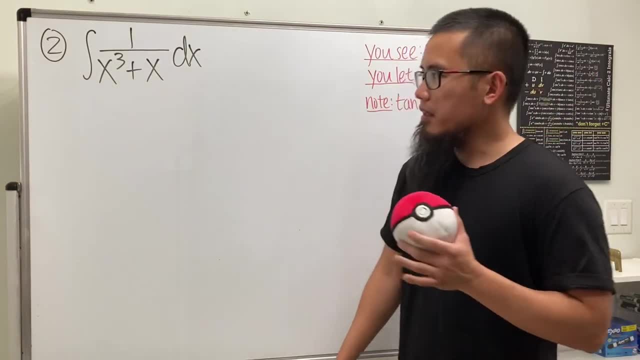 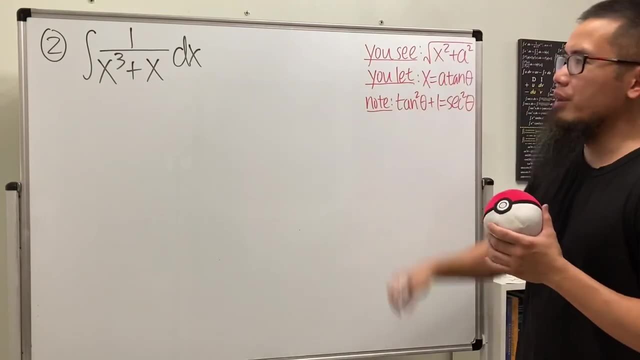 video. so we will do tricks up, But the thing is that you see, we have x plus third power plus x. That's not what we have right here, huh. So this is what we are going to do: Just factor out the x and see what happens. 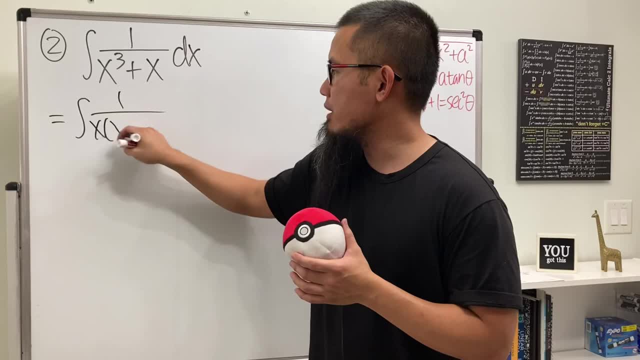 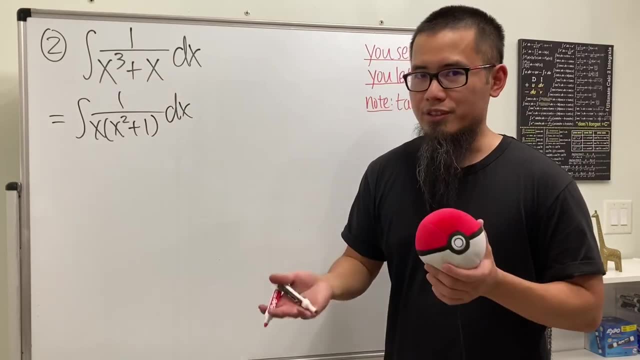 Integral 1 over, I will factor out the x, and we are looking at x squared plus 1 inside, and then we have the dx. From here we can do tricks up Here. the a is 1, we'll just go ahead and say x equals 1 times tangent theta. 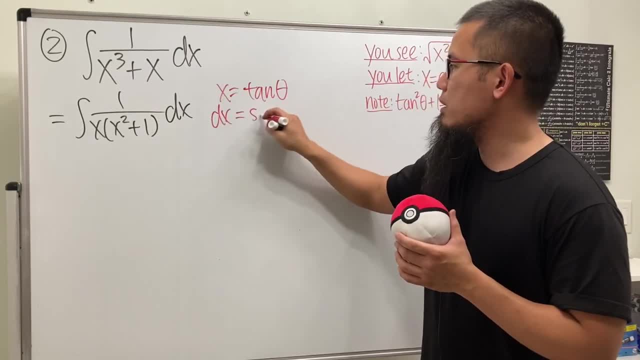 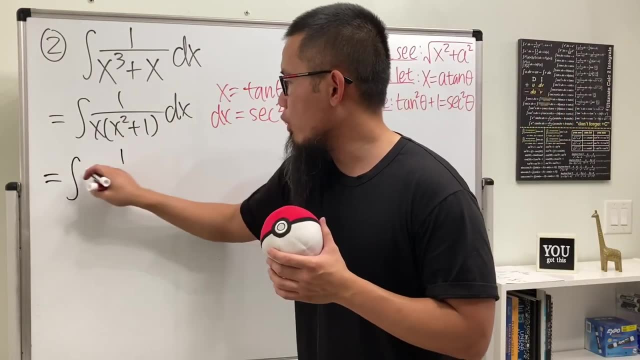 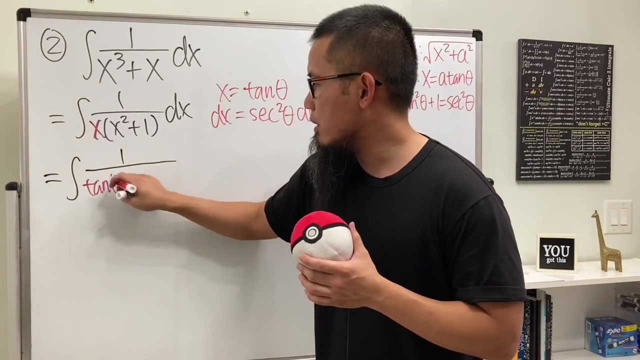 and then the usual business, dx is just going to be secant, squared, theta, d theta. Okay, here is the integral. We have 1 over here. we have x, which is tangent theta. so let's put that down And, if you are comfortable enough, 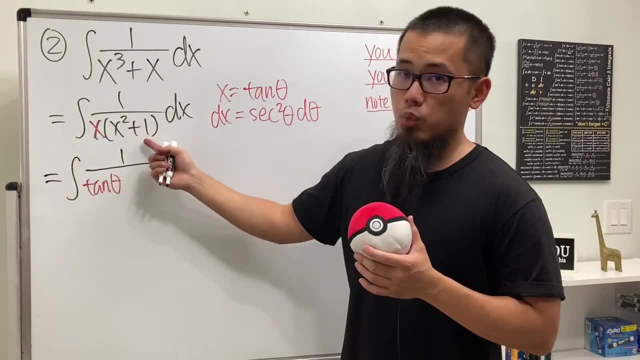 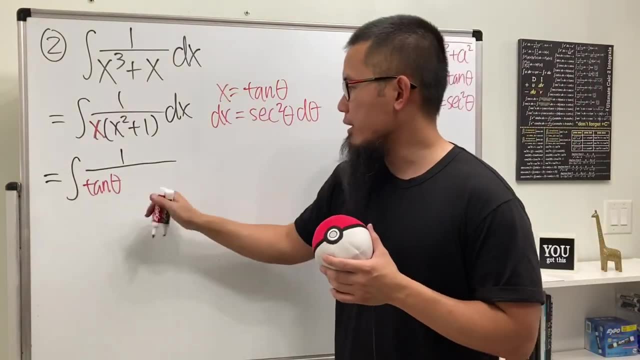 you see tangent squared theta plus 1, you know you can just put down secant, that's fine. but I want to do this work for you guys, So let me just rewrite it right here so you can see the substitution. Here we have x and that's tangent theta. 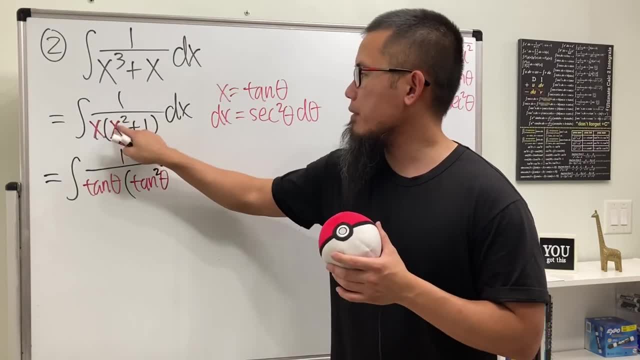 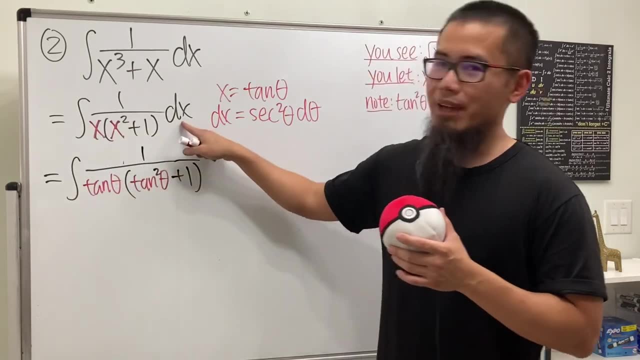 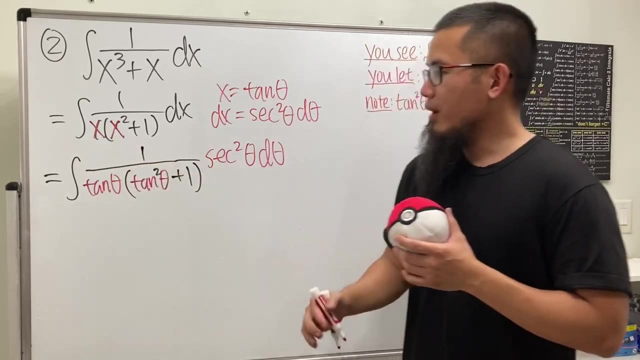 but we have to raise that to the second power and then plus 1.. All right, so that's good. And then we have the dx, which is that: so let's put down secant squared theta, d theta. Okay, Let's see, this is equal to secant squared theta. 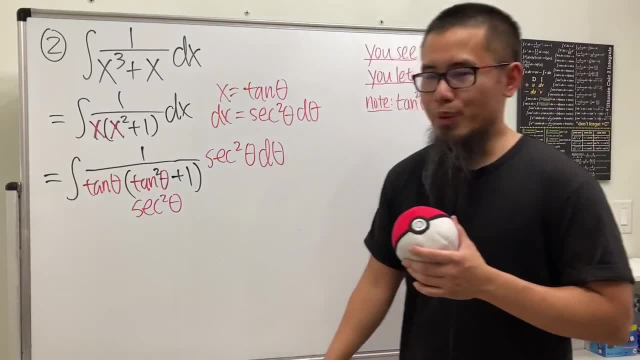 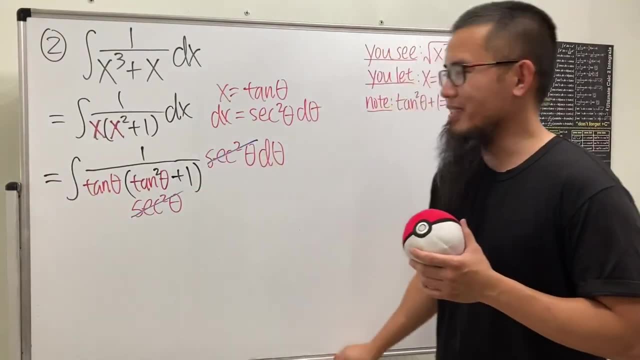 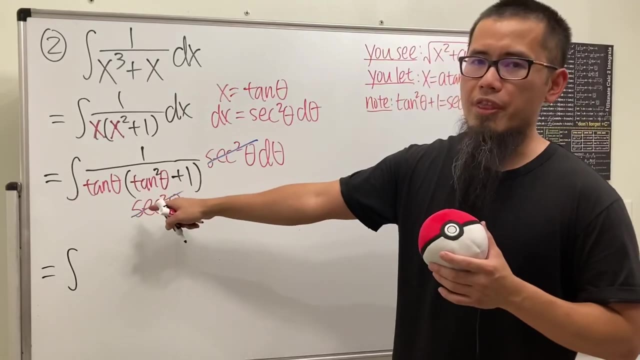 so let's put that down, Well. well, we see that here we have secant squared theta and that's also secant squared theta, so they happen to cancel each other out. Here we are looking at the integral and we have 1 over tangent theta. 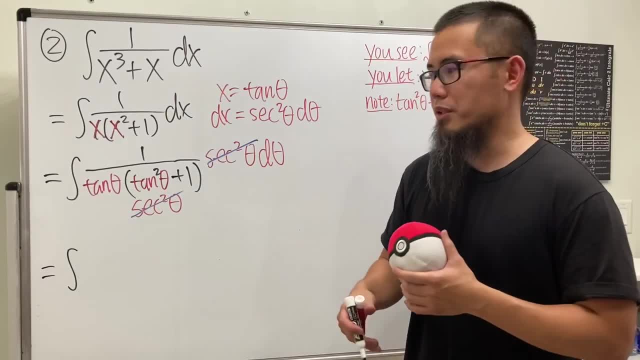 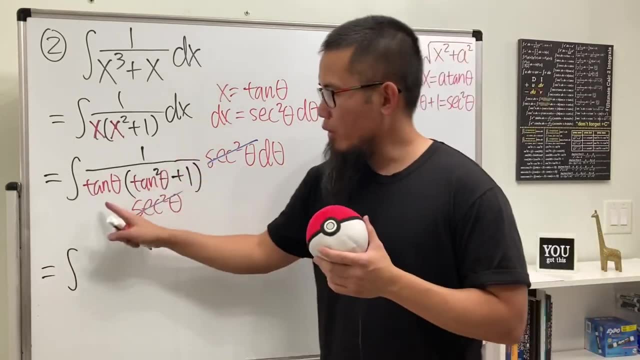 It's just cotangent, and if you know the standard result, you can just go ahead and put down the answer. but let me just do that for you guys: 1 over tangent, it's the same as cotangent, which is cosine over sine. 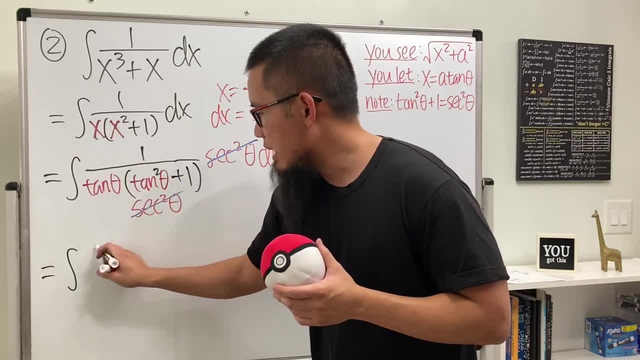 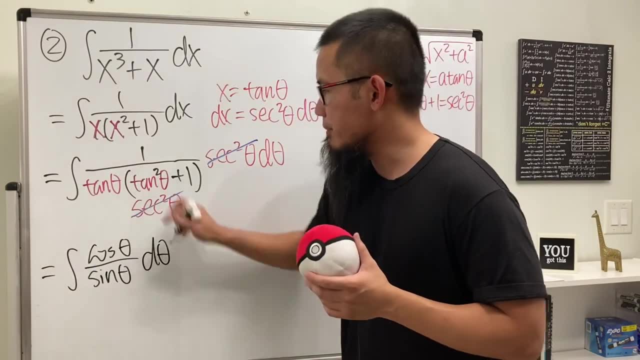 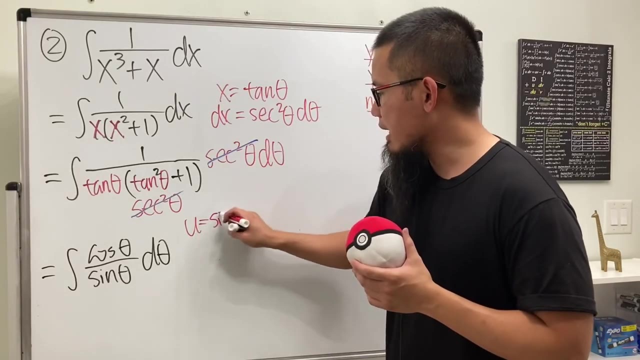 so I'm going to look at this right here and put down cosine theta over sine theta, and then we have the d theta here, Okay, So right here I can just do a? u sub that u equal sine theta, and then you see d? u equal to cosine theta d theta. 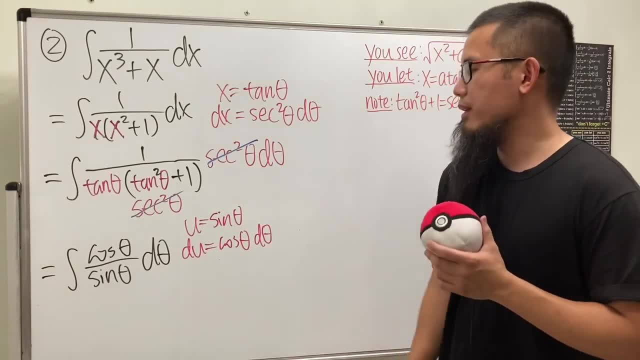 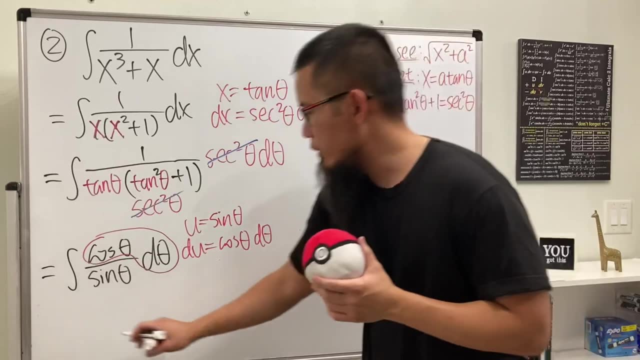 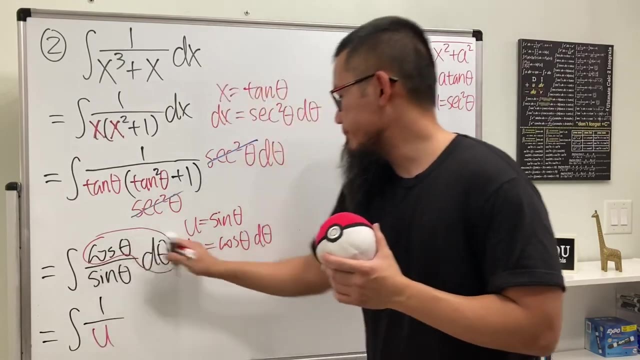 So this is the regular? u substitution and we can take this to the? u world. You see that this right here is precisely our d? u. so we are looking at: the integral of 1 over sine is the? u and then this part is the d? u. 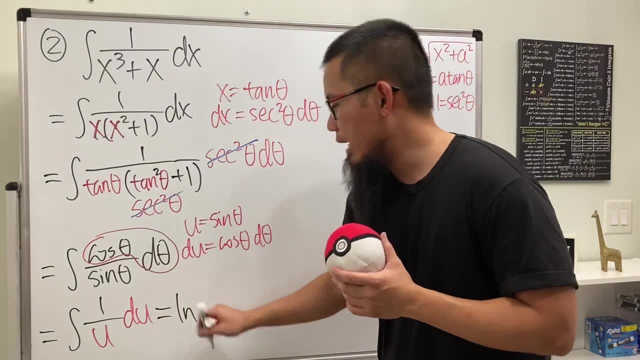 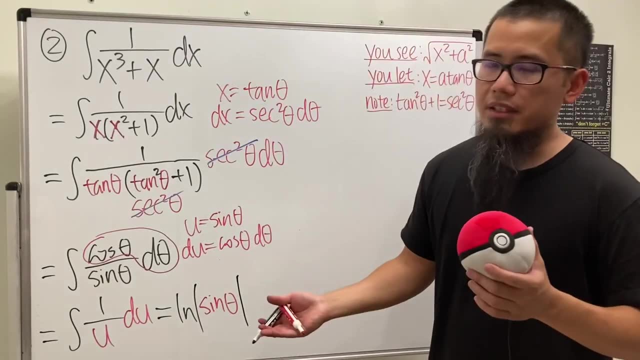 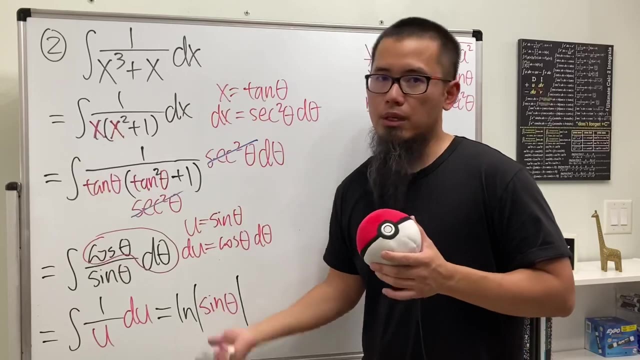 So of course we just get ln. absolute value of u and u is sine theta, so we can just put that down. and again, as i said earlier, if you recognize we are integrating cotangent theta. you could have gone from here to here, but i just want to do the little proof for you guys, just in case if you need to see it. 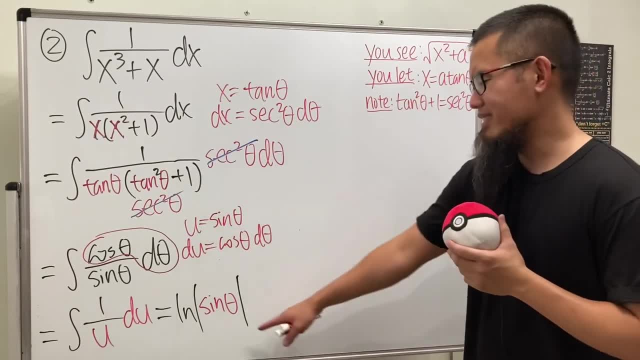 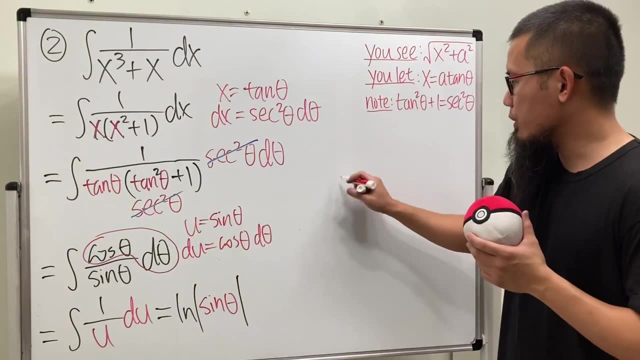 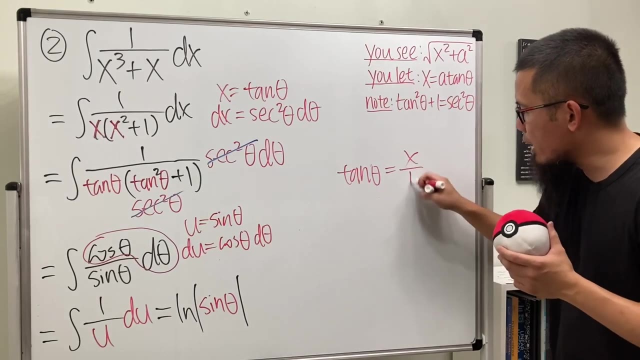 we're not done yet, because this is still in the theta world, so we have to go back, and to do so, we are going to look at this. so here we know that tangent theta is equal to x, and we are going to purposely look at this as x over one, so that we can draw our right triangle. 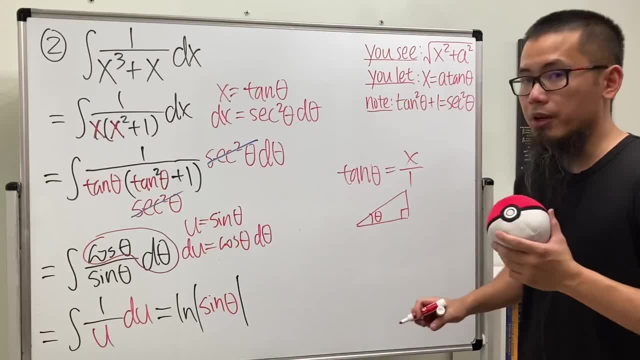 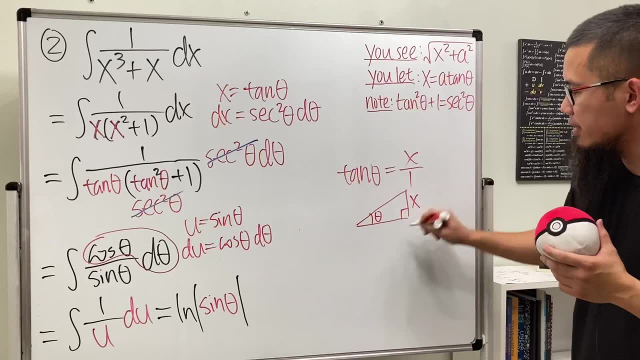 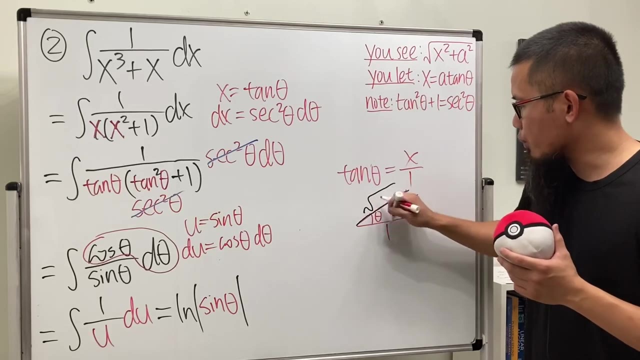 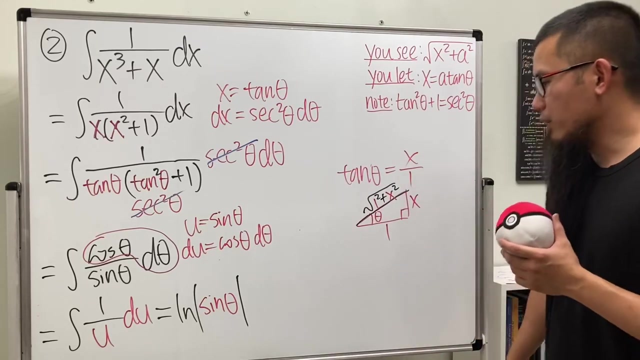 put the triangle here and then the angle theta. here, this time we have tangent, and that means we have to do opposite over adjacent. so it's like this. and now to figure out the hypotenuse: first you open the square root and you this thing square, and then you do that thing square, yeah, just like that. so finally, what do we? 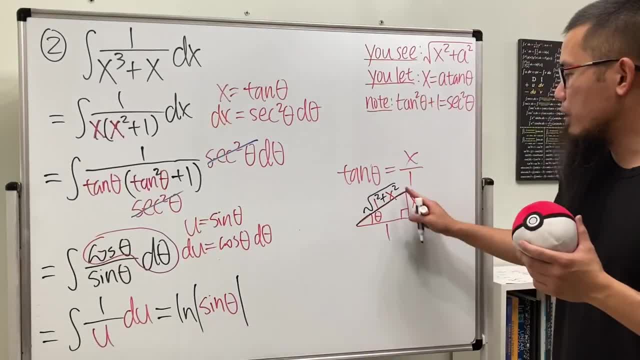 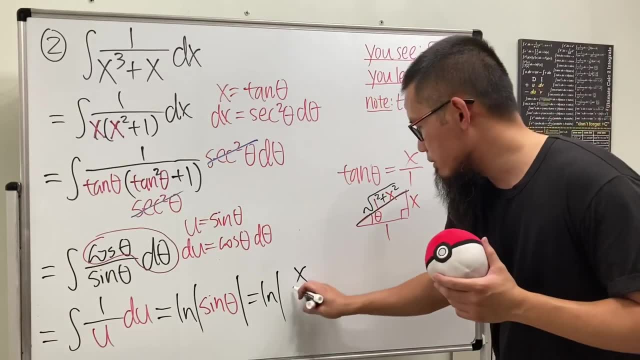 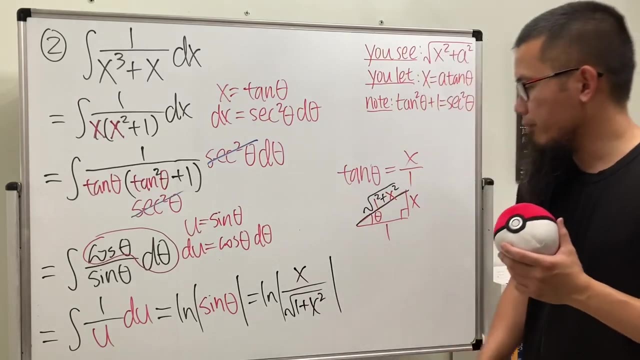 have sine theta is just opposite over hypotenuse. so all in all, we can look at this as ln absolute value, and we have x over that, over square root, and we have one square which is one, and then the x square. yeah, just like this, and then we are done. put a plus c. 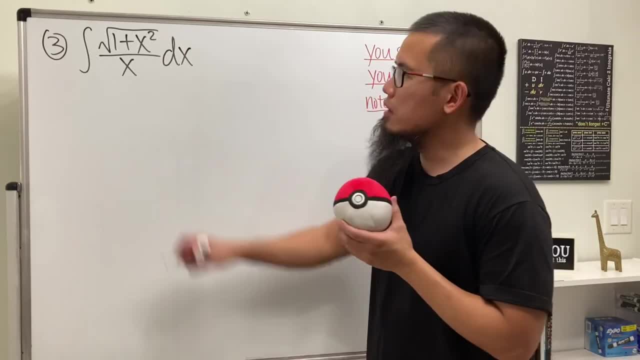 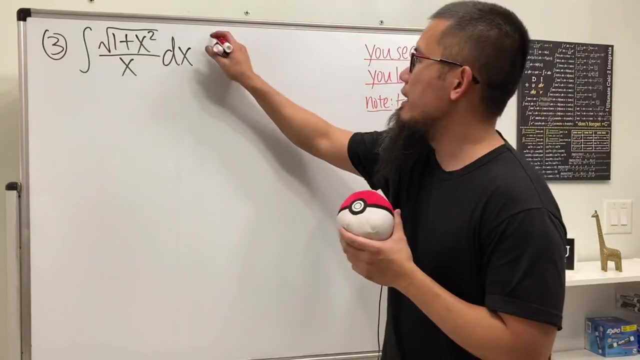 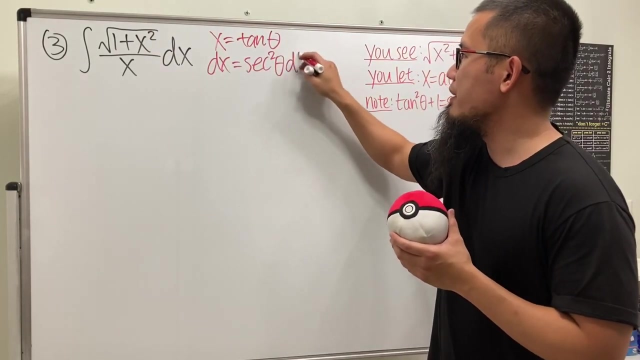 this is it for number three. we have the integral of square root of one plus x square over x. so we see the a is equal to one. let's just get started that x equal tangent theta, and then dx is just secant square theta, d theta. in fact, this is the hard one, and you'll see why. 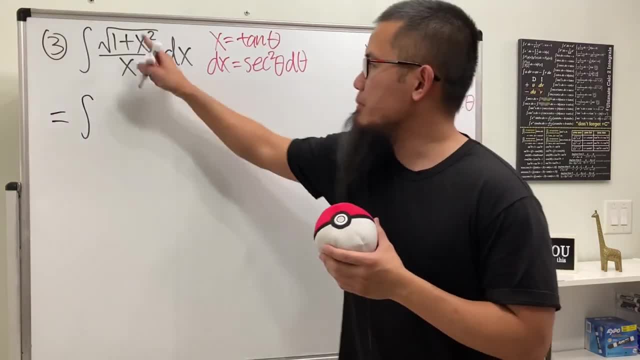 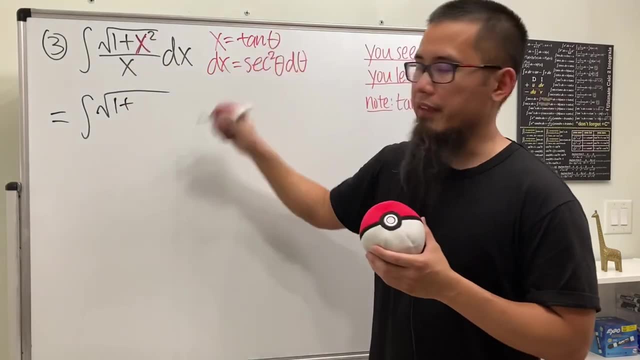 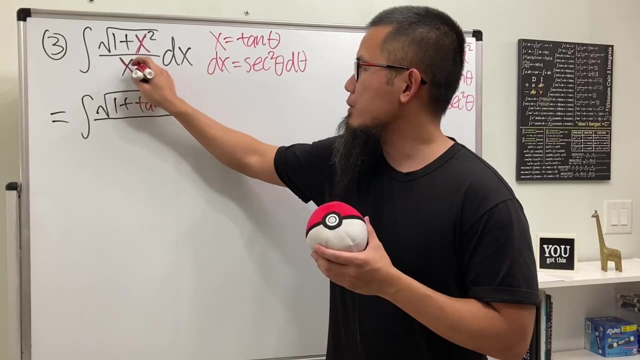 so let's see, here we have the integral and i'm just going to put down square root, and we have one plus, and this is the x which is tangent theta, and then we will have to square that. so i'll put a square right here and then over another x which is tangent theta, like this, and then for the dx we have that. 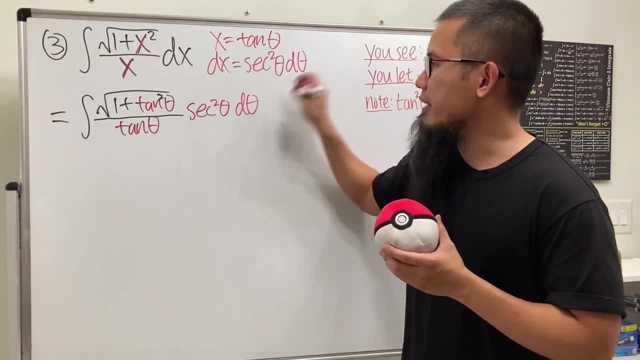 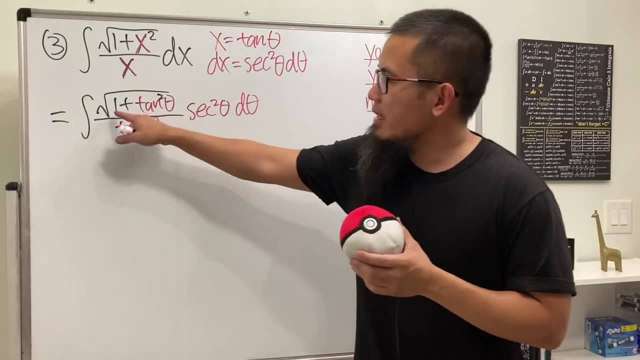 so we'll put down secant square, theta d theta. all right, so now perhaps we have done this enough already, so we can do a little bit of this, and then we have to do a little bit more of this. now let's do a couple of them in our head, this right here is just secant square, but that's inside the square. 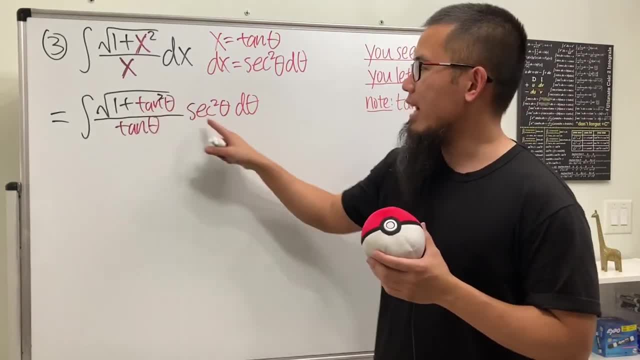 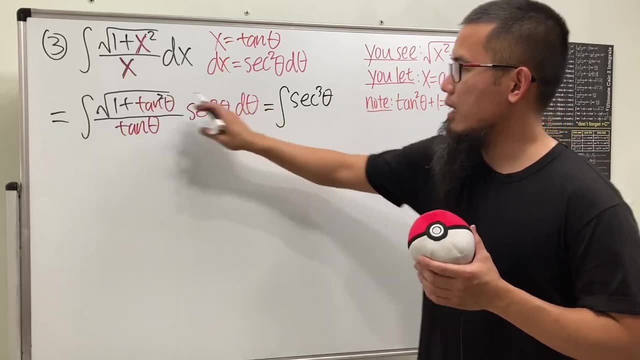 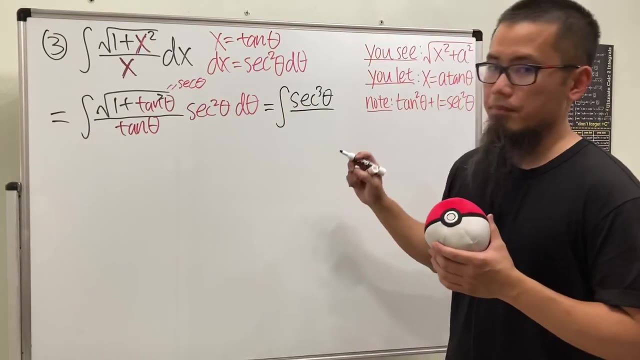 root. so we just get secant theta right and we have another secant square theta. so all together it seems like we have secant to the third power theta on the top right again. all this right here is just equal to secant theta. and then on the bottom we have tangent theta, so that looks okay. 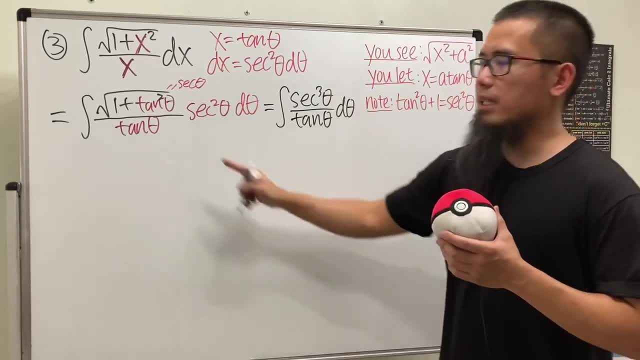 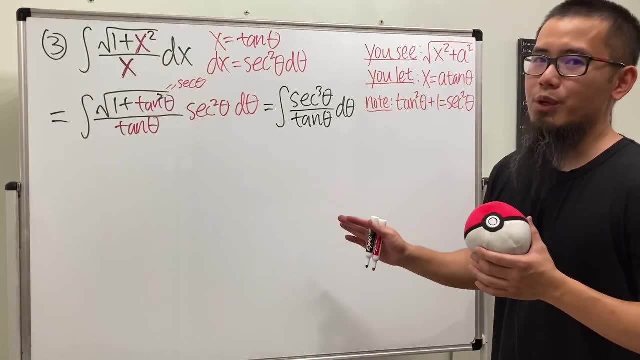 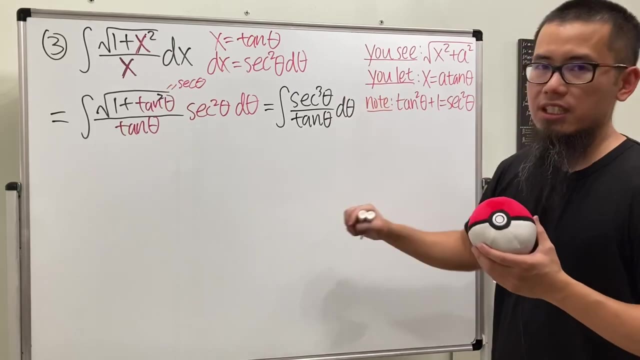 right, just multiply this and that we get this and then we have the tangent theta on the bottom. but the thing is that i think this right here it's actually kind of hard to integrate. so you guys can let me know. maybe some of you guys would prefer to write everything in terms of 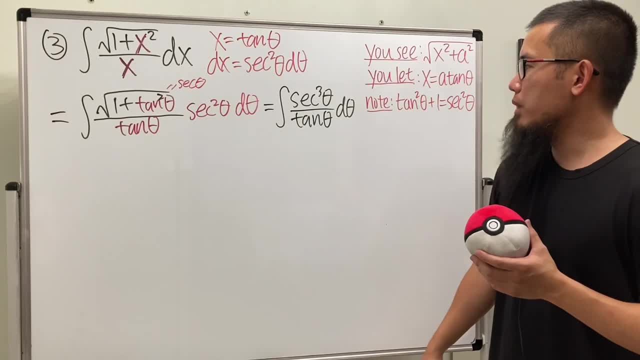 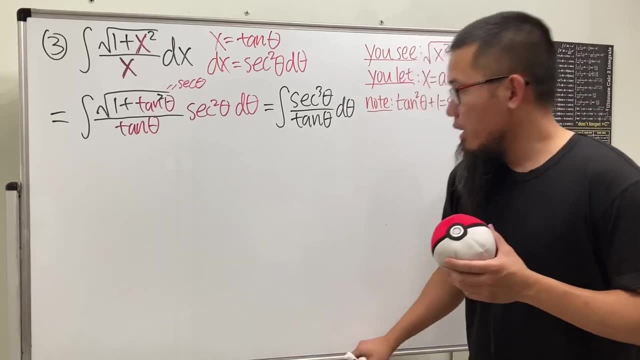 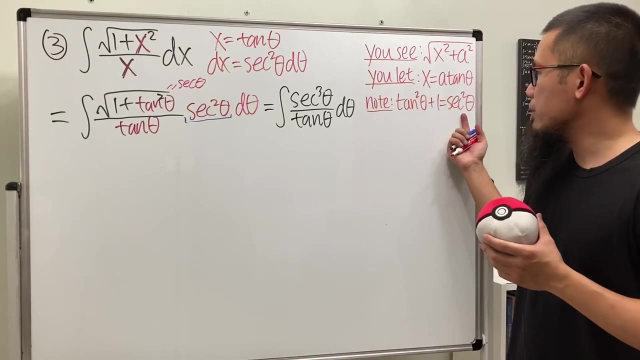 sine and cosine you. that might work. or maybe you have any kind of way to do it, you can let me know, but this is how i would like to do it. notice, here we have secant square theta. what i will do is we are going to actually look at this. 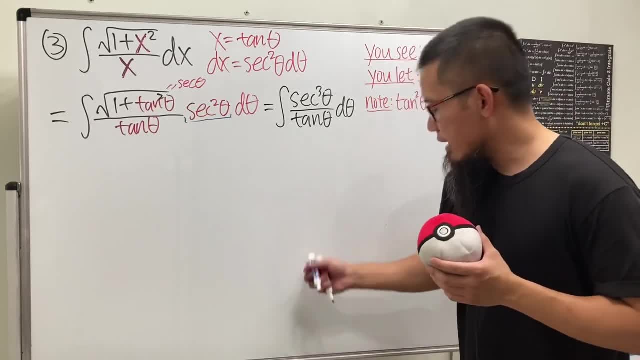 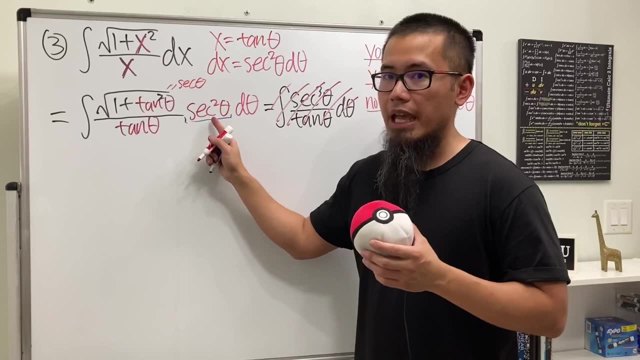 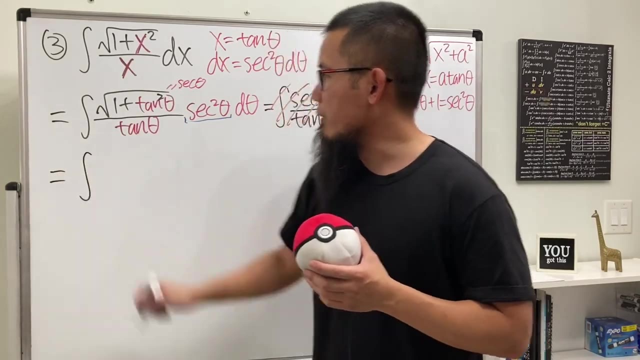 backwards and you'll see why. so again, i am not going to continue right here because of the secant to the third power. i'm going to utilize this and i'm going to uh, you, you, a break it apart for you guys. so here is the deal. we have the integral. 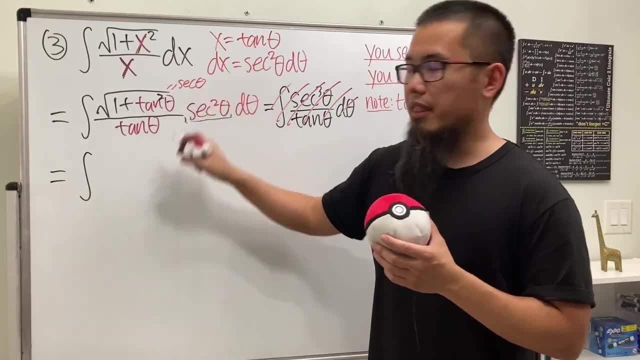 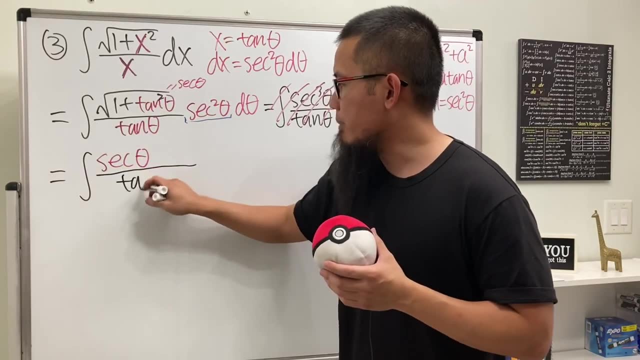 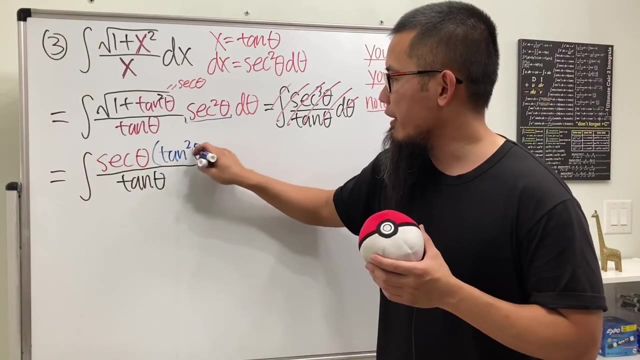 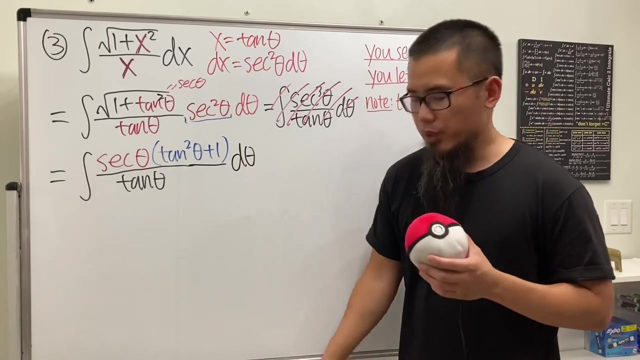 we have a secant theta on the top, so let's put that down and then over. this is tangent theta on the bottom, so no big deal, but for this part i will rewrite this as tangent square theta plus one and we are in the theta world like. so why do we do it? because the 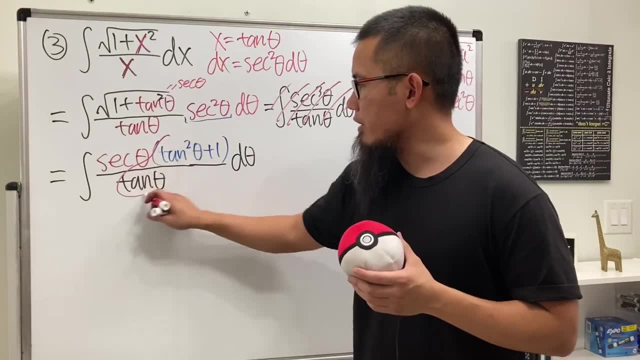 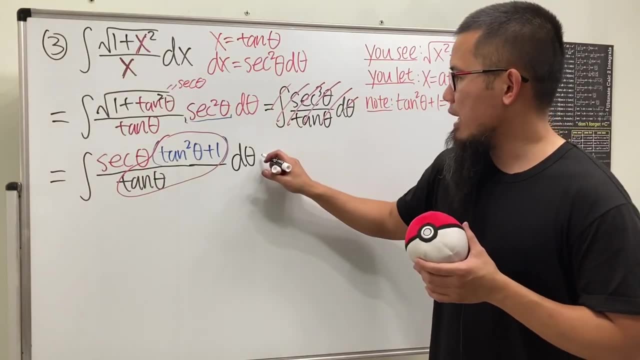 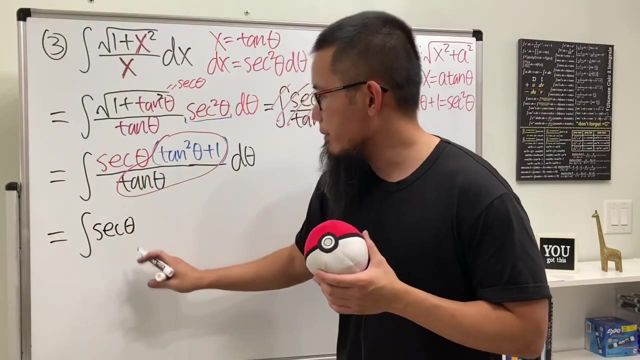 this way. i'm going to just pair them up together and you'll see they simplify pretty nicely. have a look right here i'm just going to write it down. right here we have the integral: this is secant theta in the front right here. well, you see, we have two things on the top over tangent theta, so you can just do this over that. 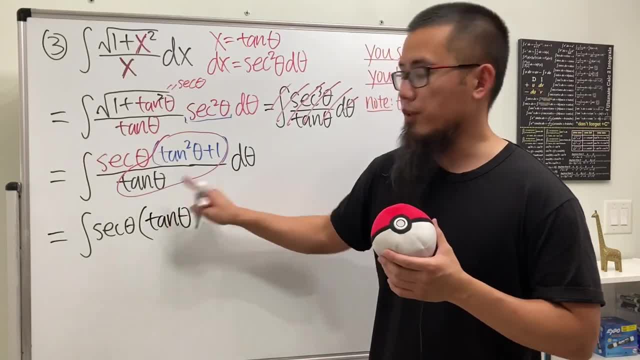 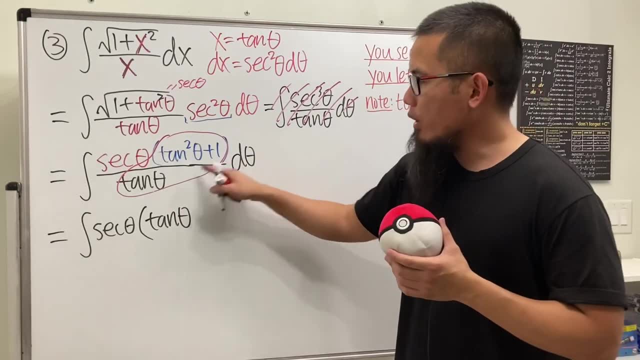 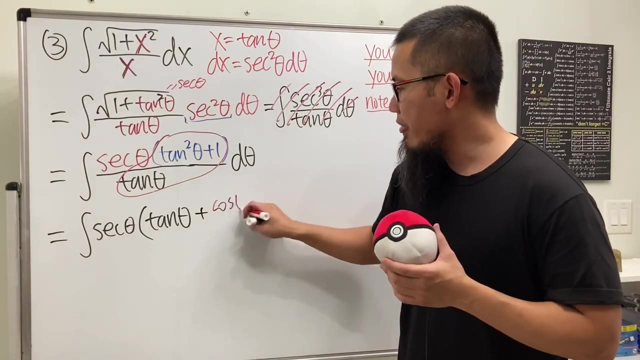 and that will give us tangent theta and that's tangent to the first part. right this over that. Next, we have 1 over tangent theta. 1 over tangent theta is the same as saying cotangent, which is just the same as saying cosine theta over sine theta. 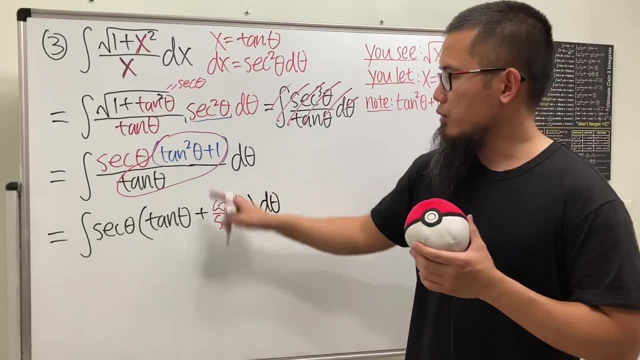 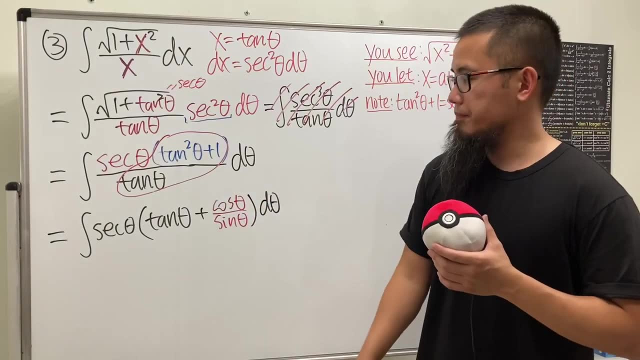 And then, of course, put on the d theta right here. So again, 1 over tangent, theta is just cotangent, which is cosine over sine, And that's what we have. Okay, here is the deal. I'm going to multiply this in. 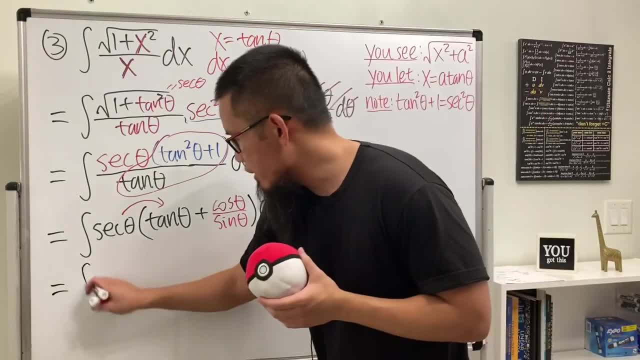 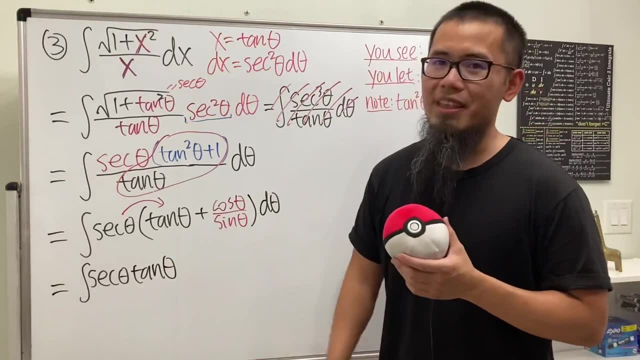 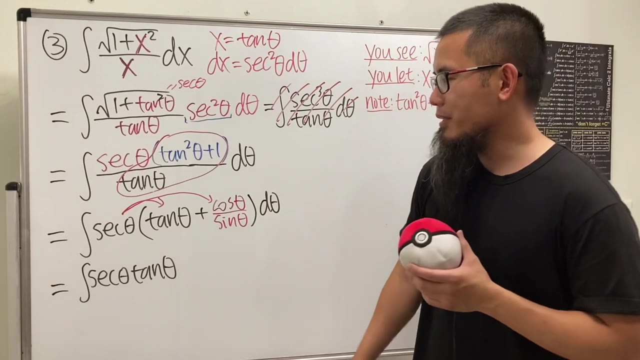 And we see that the first part is actually nice because we can integrate secant theta times tangent theta with ease, because the answer is just secant theta. But when we multiply this and that, well we actually have to recognize that secant theta is the same as 1 over cosine theta. 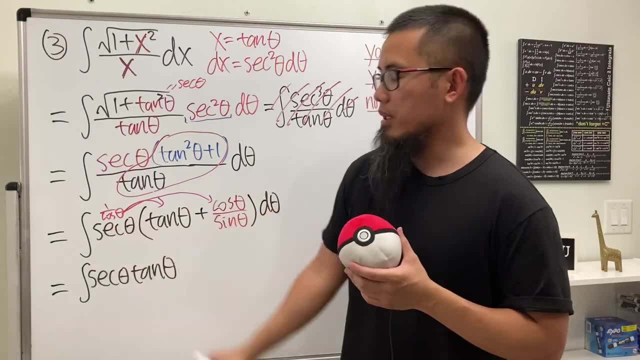 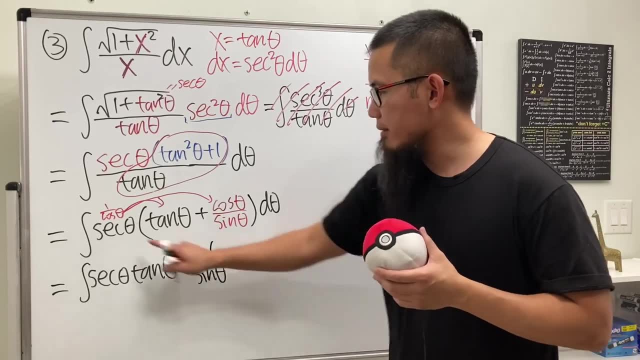 So when we multiply this and that, the cosine theta will cancel out, In fact we just increase And that way it's plus 1 over sine theta, because again they cancel out. And I'm just going to replace this with what. 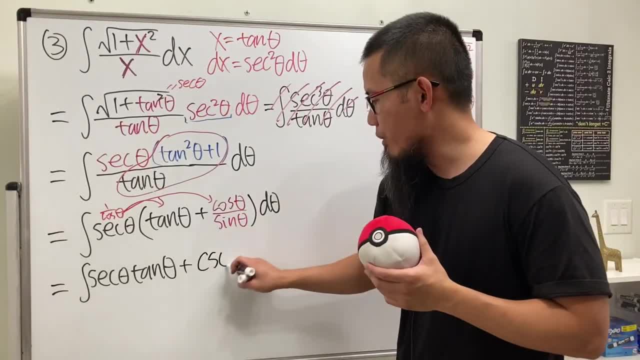 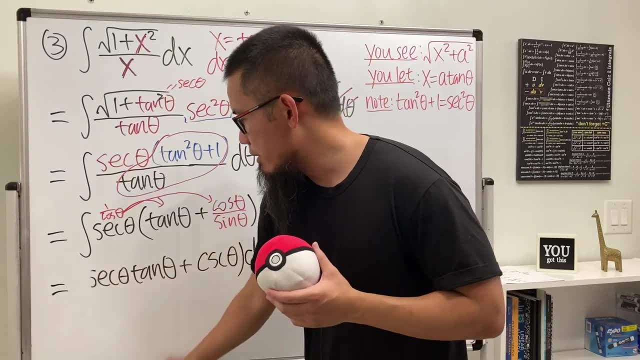 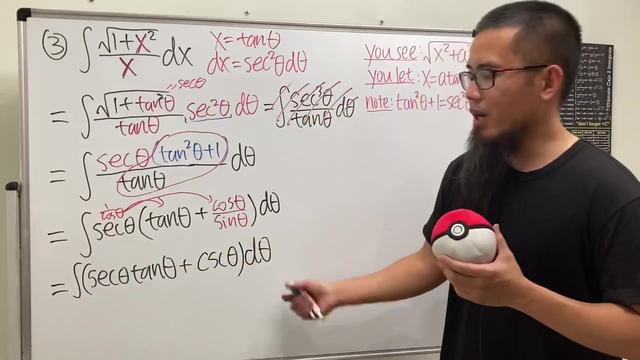 Cone secant theta. Yes, So this is cone secant theta like. so d theta like this, And then perhaps I'll put on the. A lot of people really want me to put parentheses right after the integration sign, before the d, whatever. 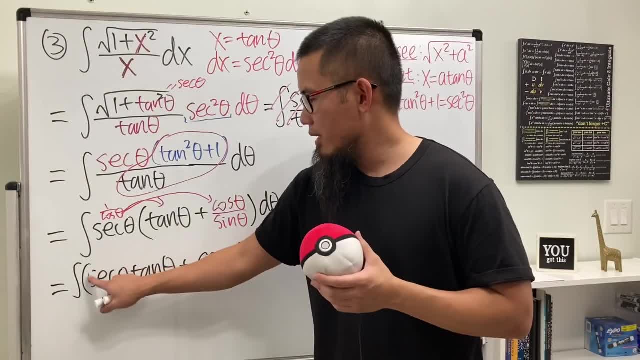 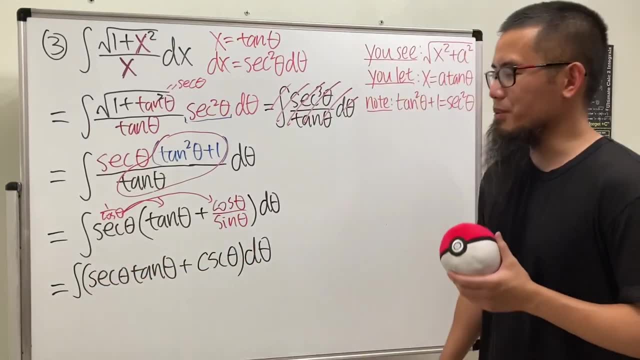 Uh, sometimes, Sometimes I do, Sometimes I don't. Why do I do it? Technically I should, But why don't I do it? I really think it's clear. So anyway, I don't really mind. But anyway, this is pretty much the prep work that we'll be doing, right. 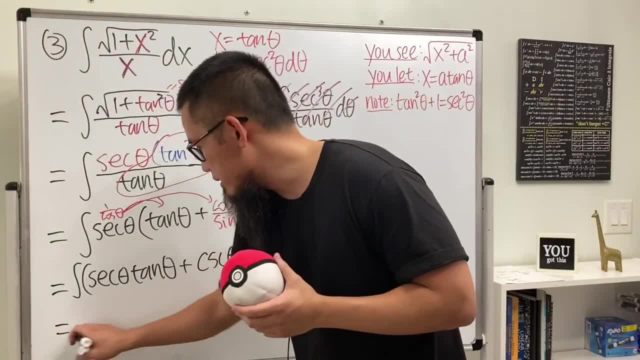 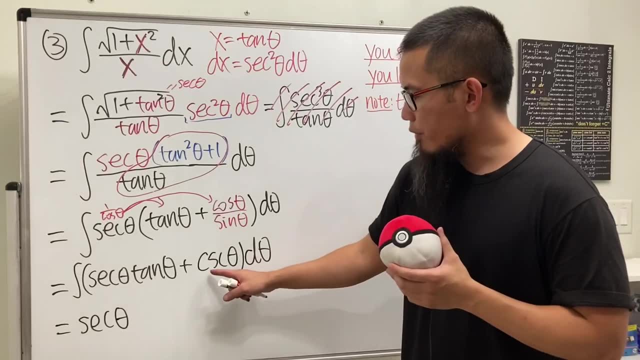 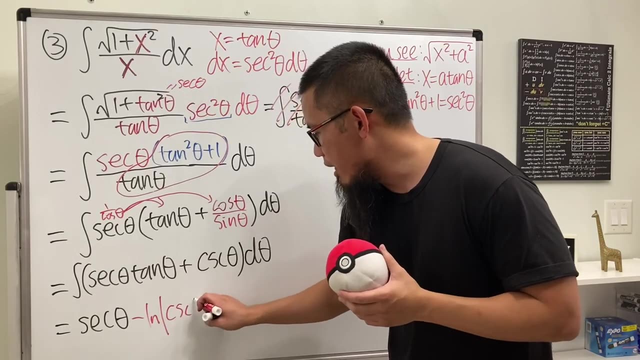 And now we can integrate this pretty easily because that's just secant theta And we are done. But for this we have the integral of cosecant theta. I will be using this answer, Namely negative Ln, absolute value, cosecant theta plus cotangent theta. 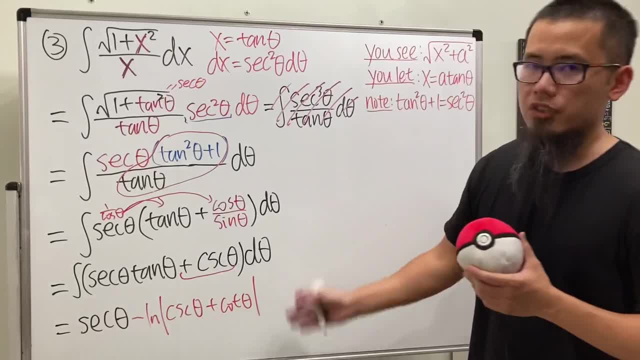 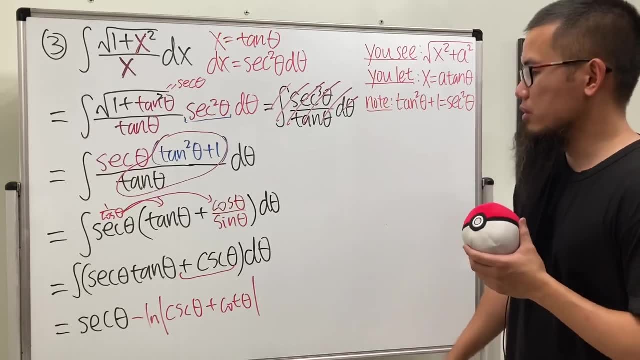 All right, So this gives us that You guys can check out my other video for this if you guys need to. Okay, Now the rest of the work is just go back to the x world, So we are going to refer back to that. 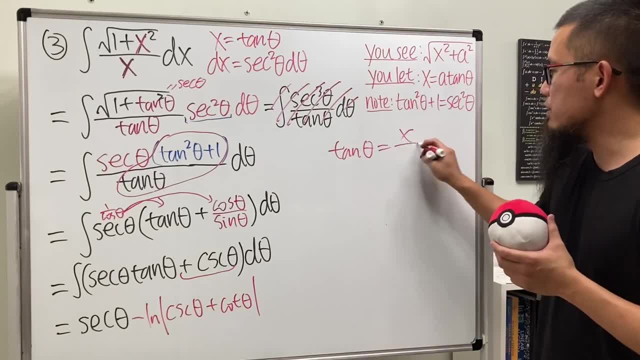 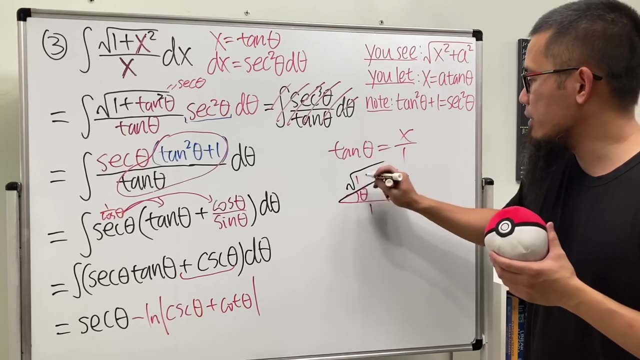 So we're looking at tangent. theta is equal to x, which is the same as x over 1.. Draw the right triangle, Put the angle here. X is the angle Opposite, 1 is the adjacent Hypotenuse, is square root of this guy plus that guy and both of them. 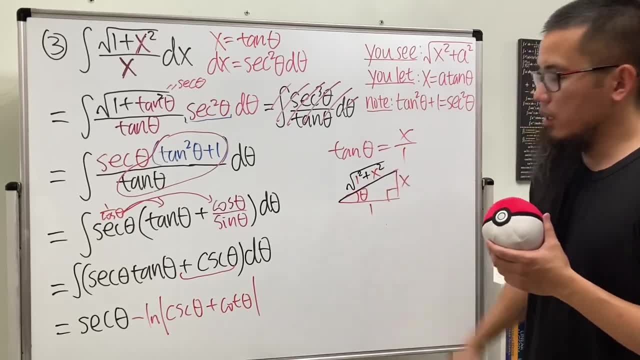 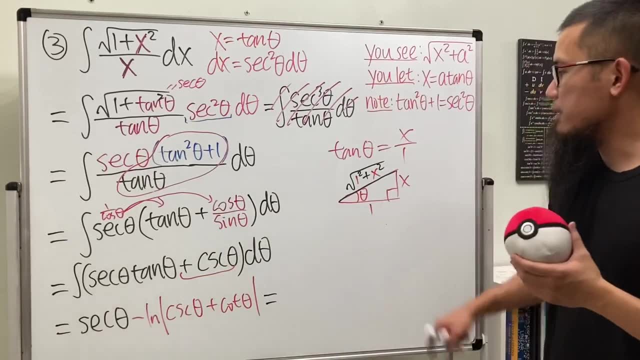 to the second power individually like. so With this we can figure that out. Check this out: Here we have secant theta. Secant is hypotenuse over adjacent, So we just have that. So that's the first part. 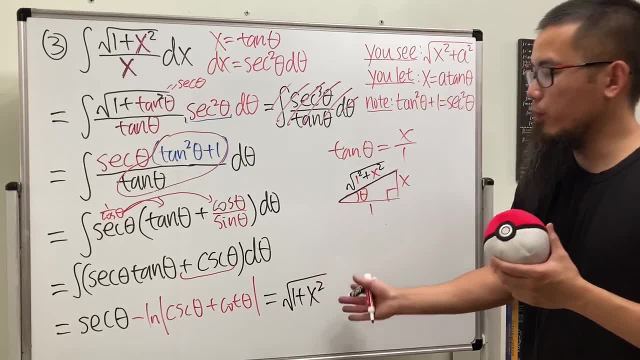 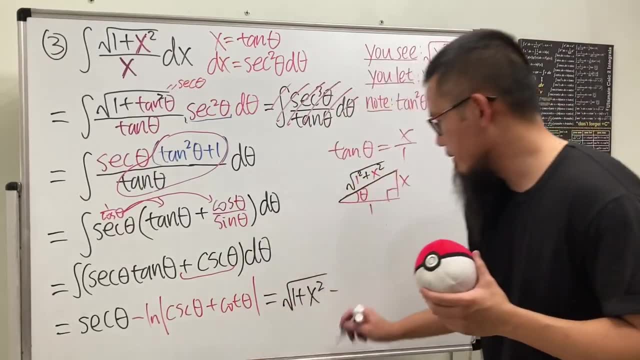 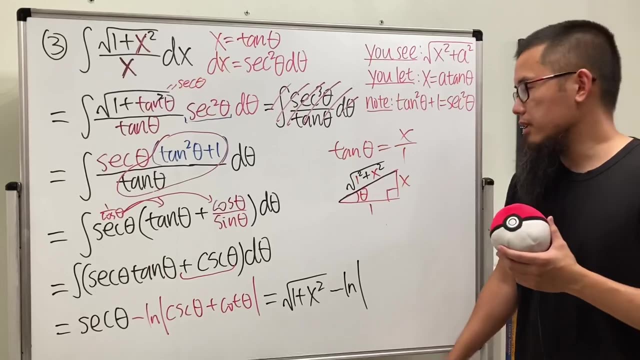 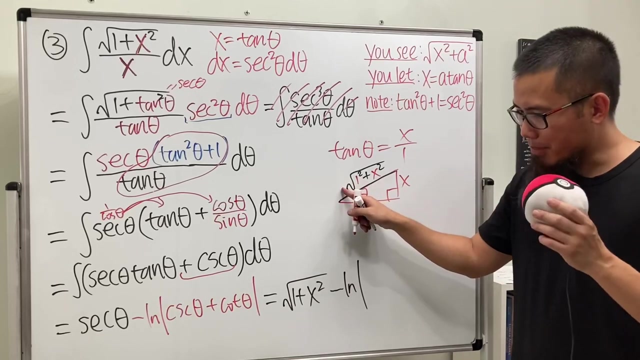 Square root of 1 plus x squared, And we are done for that. Next we will have the minus, and perhaps I'll change this to, and it's okay- And then we have minus LN, absolute value, And for the cosecant theta: cosecant is the reciprocals of sine and cosecant is just hypotenuse. hypotenuse over opposite. 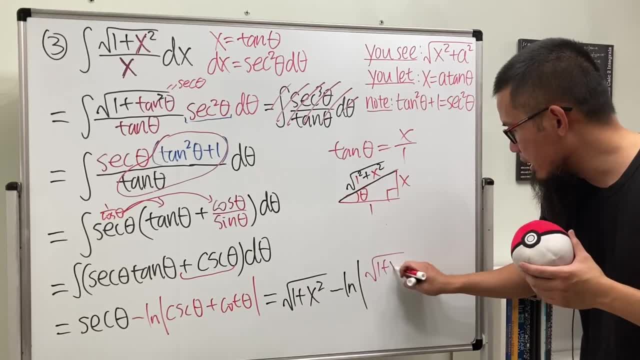 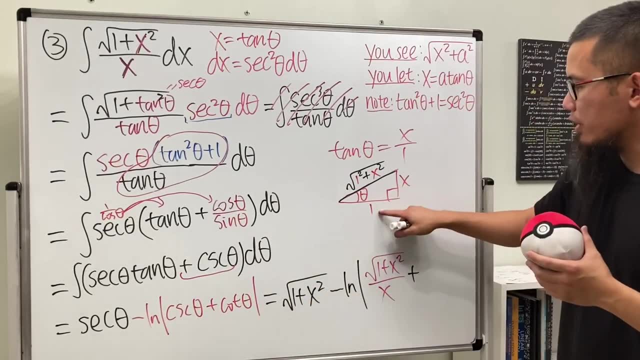 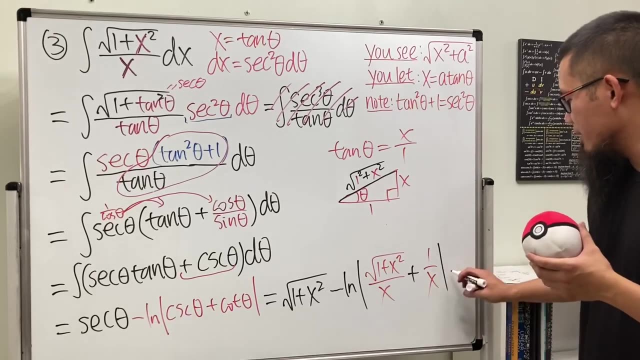 So this over that. So I will put down square root of 1 plus x, squared over x. Lastly, we add Cotangent, which is just adjacent over opposite, which is just 1 over x, And again you can put them together, but it's okay. 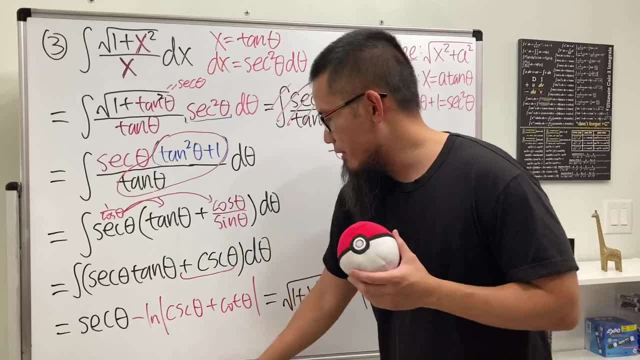 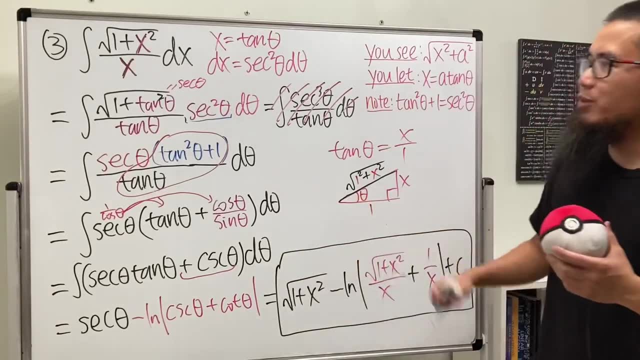 So that's all Put down the plus C, And now I think this right here, go with that. So I think this is pretty clear, Okay. So, yeah, this right here. It's a pretty hard one, So maybe you want to practice this again. 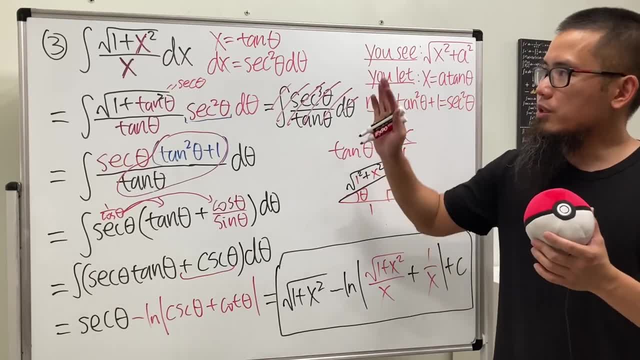 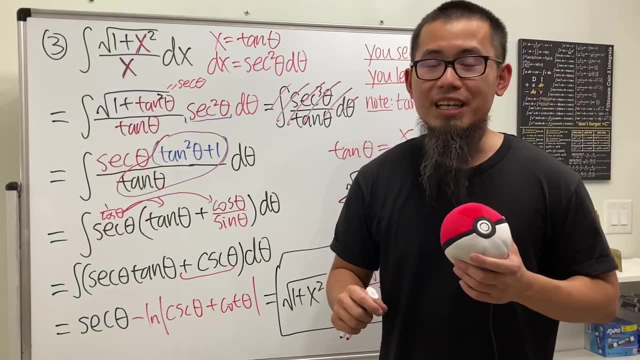 And I think the best way is you just just just write this down again on a sheet of paper And then try to see if you can redo everything by yourself or not. Don't look at any notes, And if you can really do it, that means you are getting it. 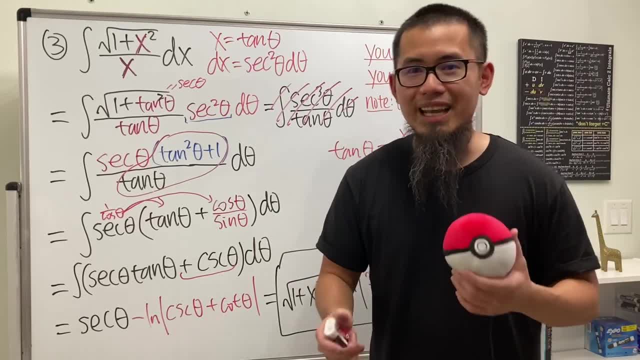 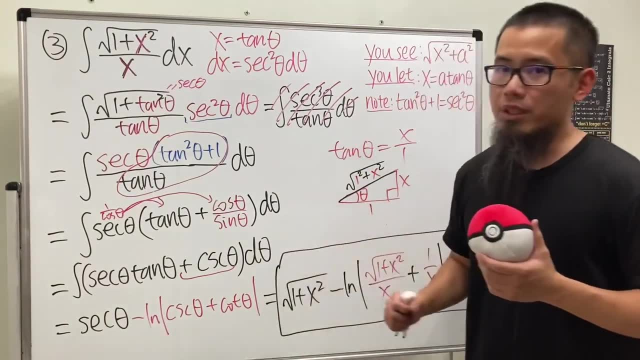 And you will build up the confidence when you are able to do it, And that's what you really need in order to be successful in Cal 2.. And, of course, if you get stuck, then just take a look of what we did again. 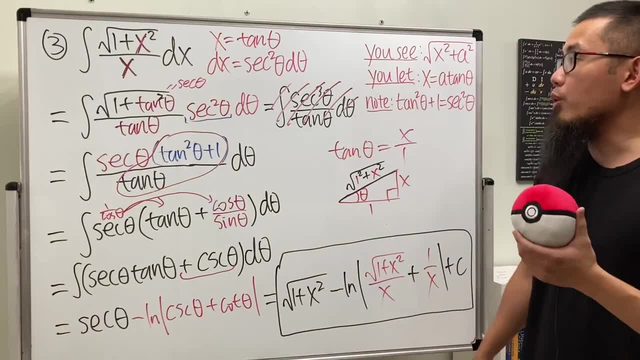 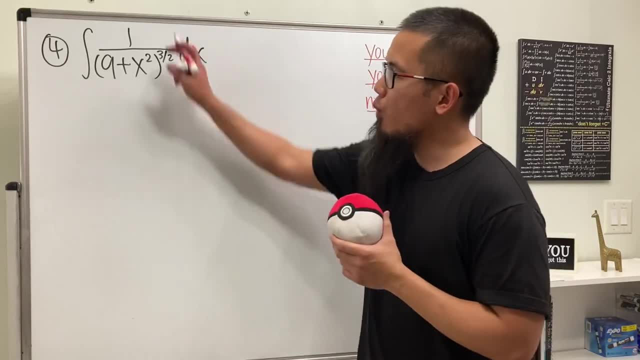 And then just try to practice on your own. Yeah, So for number 4, we have 1 over Number 4, we have the integral of 1 over 9 plus x. Okay, So 1 over 9 plus x squared and then raised to this 3 over 2 power. 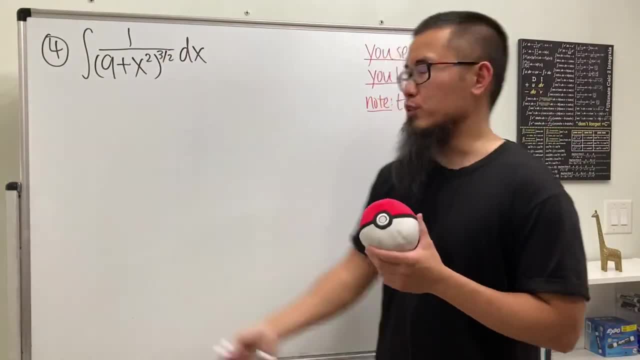 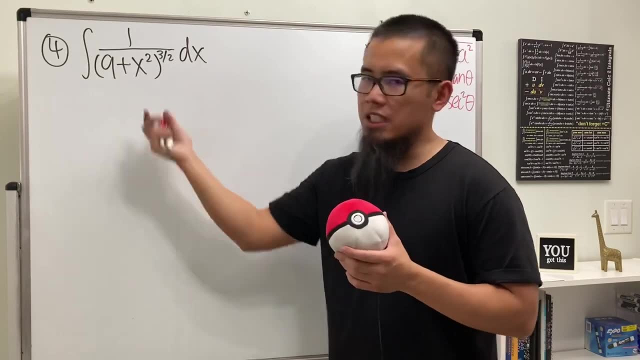 So remember, the over 2 power is the same as square root. So we are still kind of in this situation, But the main part is pay attention to that. We have two terms and we are adding: And this is the sum of two squares. 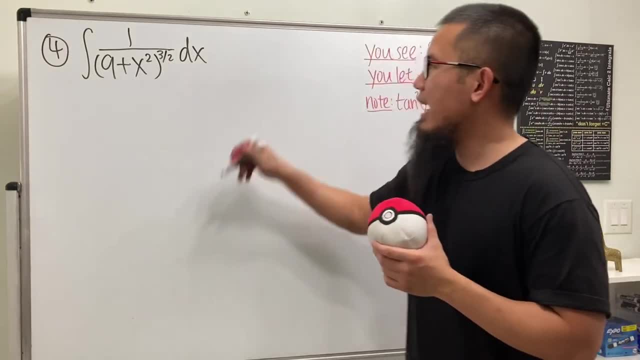 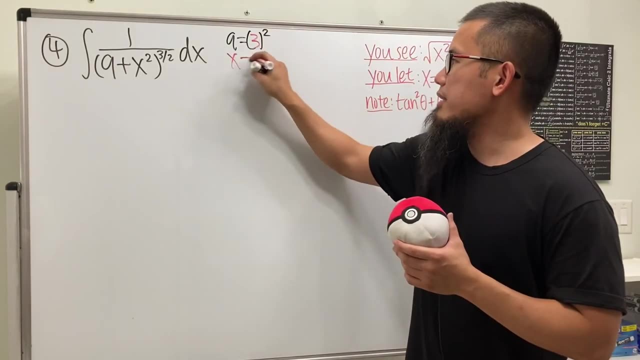 Then we use the tangent substitution Right here we see that 9 is the same as 3 squared, So a is equal to 3.. And let's begin. Let x equal 3 times tangent theta And then differentiate both sides. 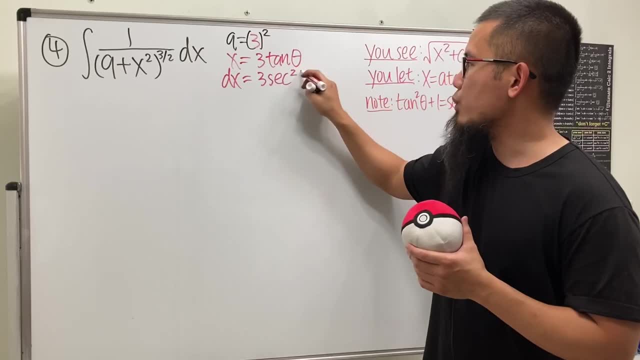 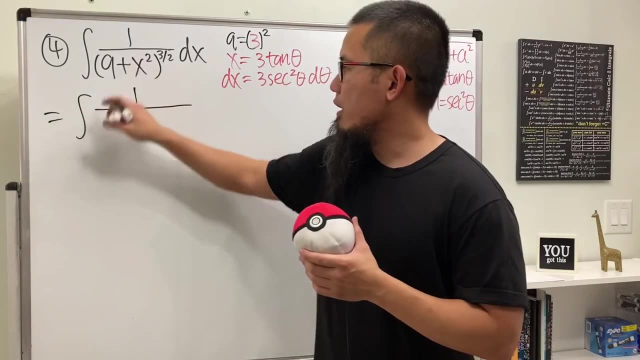 We get dx, That's equal to 3 secant squared theta d theta, Alright. So this right here is going to be the integral 1 over Parentheses. we have 9.. And then plus For this x, right here. 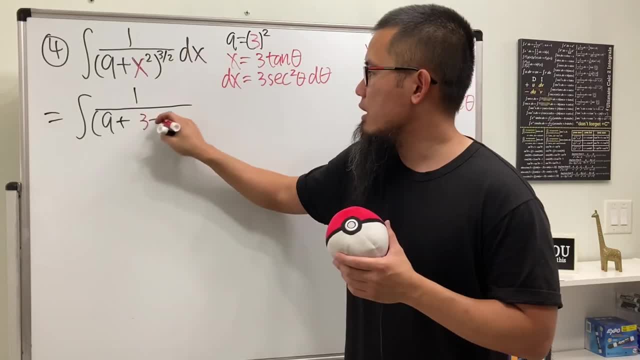 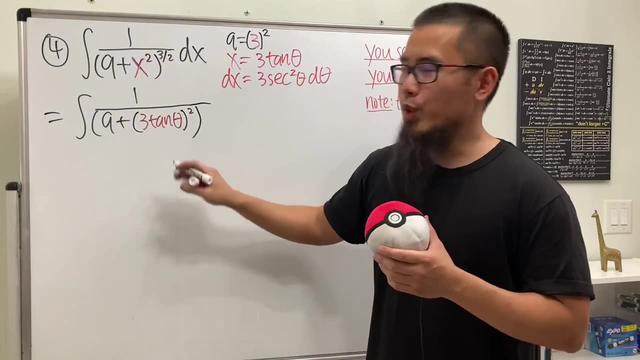 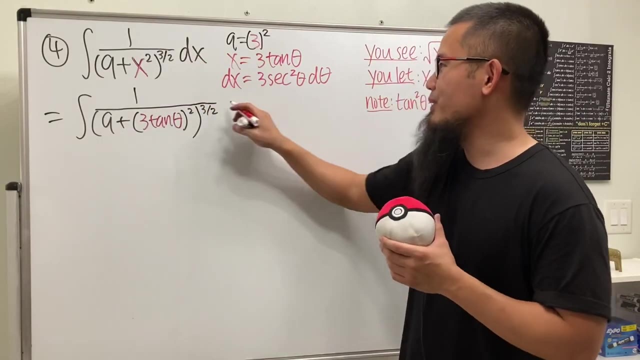 We just look at that as 3 tangent theta And then we square that And on the very outside here We will have to raise this to the 3 over 3 over 2 power And then for the dx We will write down 3 times secant squared theta, d theta. 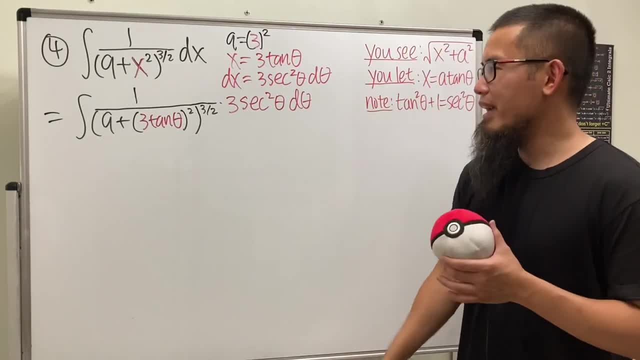 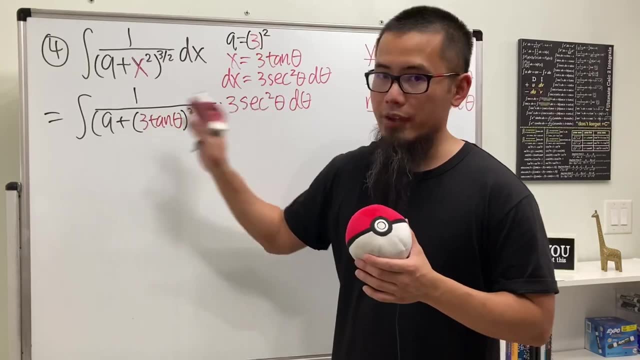 Alright, So we have this integral in the theta world And now, as usual, let's fix this part Inside out. This is 9. And this is also 9. We can factor that out. So we are looking at 9 times 1 plus tangent squared theta. 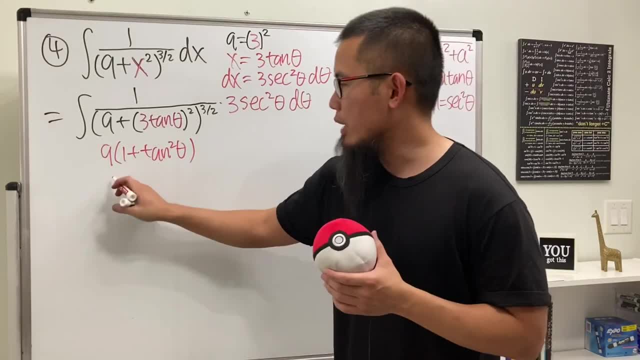 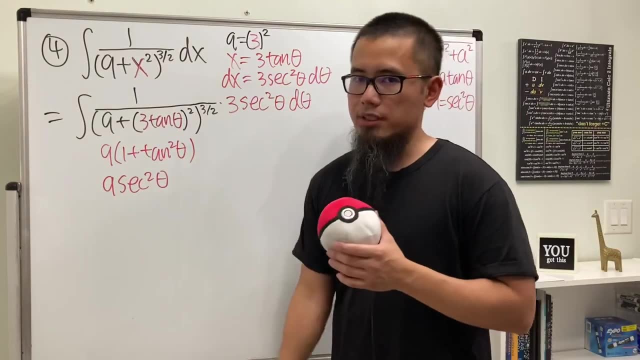 Well, this right here is secant squared theta, So we are really looking at 9 times secant squared theta. This time this is not just a square root, It's 3 over 2 power, right? So what you can do is: 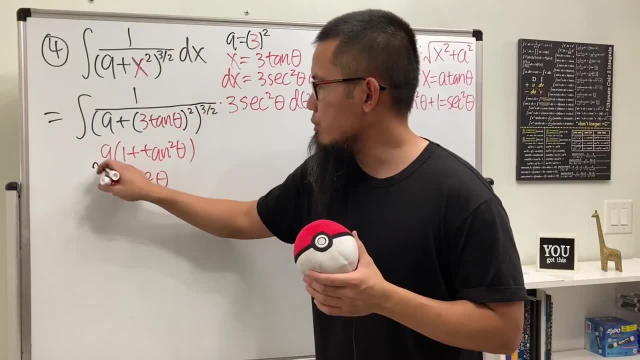 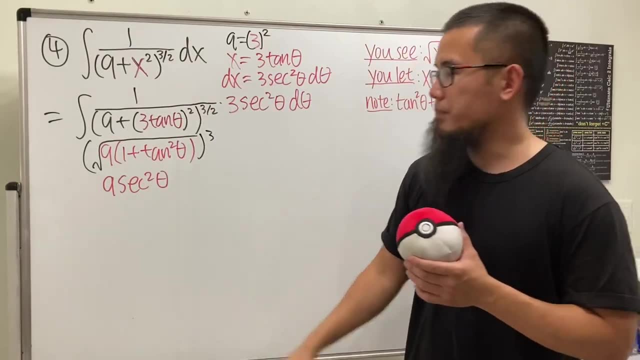 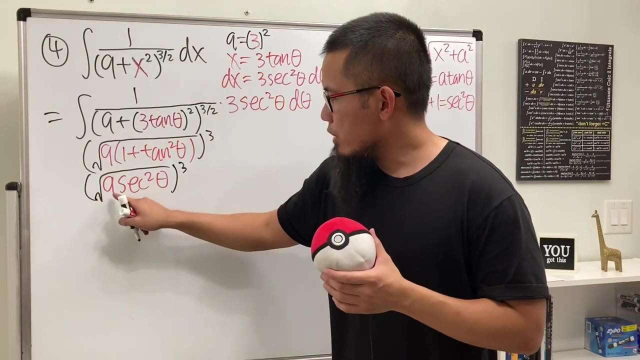 You can make the over 2 power into a square root, But don't forget to also raise the other part to be the third power. So, right here we take the square root And then we take the rest to the third power, And now square root of 9 is 3.. 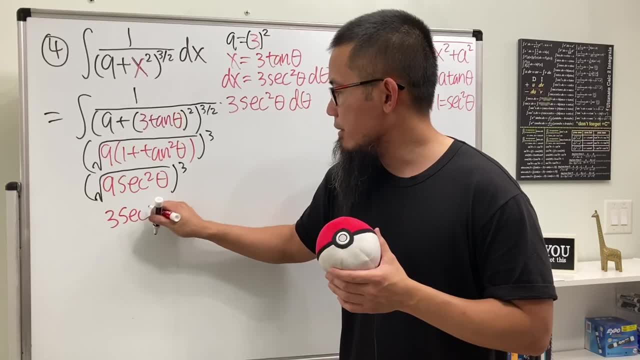 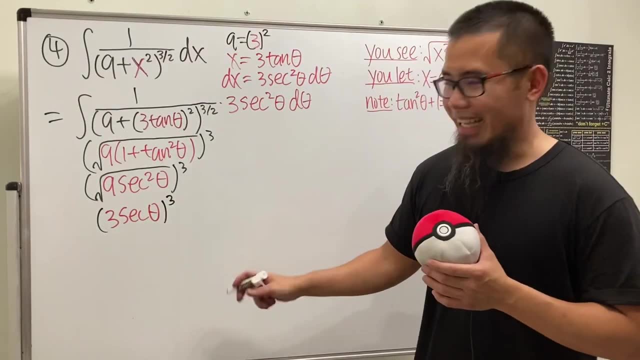 And then square root of that is just secant to the first power, And then theta, And then we have to raise this to the third power, And then this right here is 27.. And here we have secant to the third power, theta. 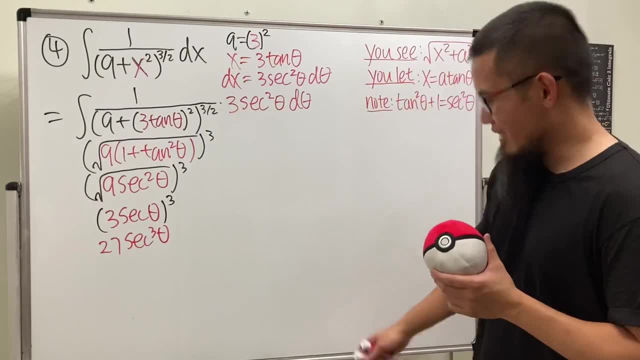 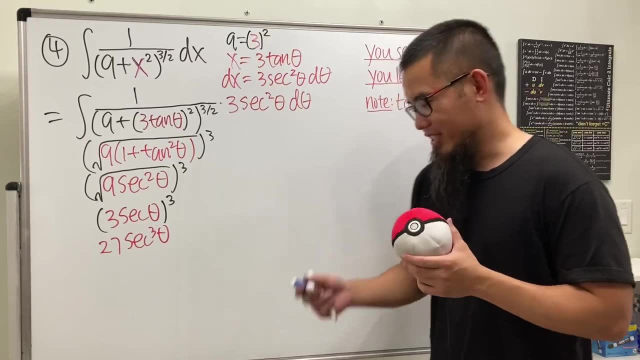 Oh, my god, That's what we have. Pretty cool, huh. Alright, Here is the cancellation part. It's actually better than number 3 in my opinion. Check this out. 3 and 27 can be reduced, So we have a 9 on the denominator. 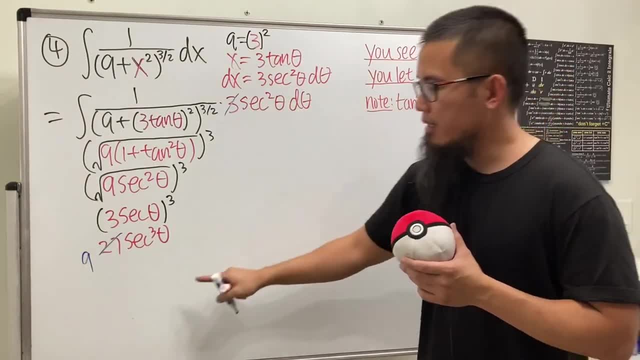 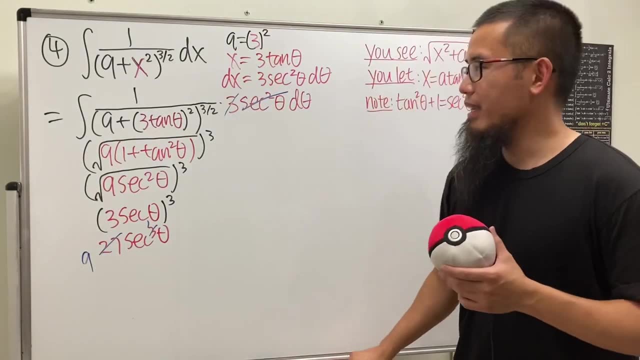 And you see that here we have secant squared, And this is secant to the third power, So we can cancel two of them out. So now this becomes the first power. So let's see what we really have. We have 1 over 9.. 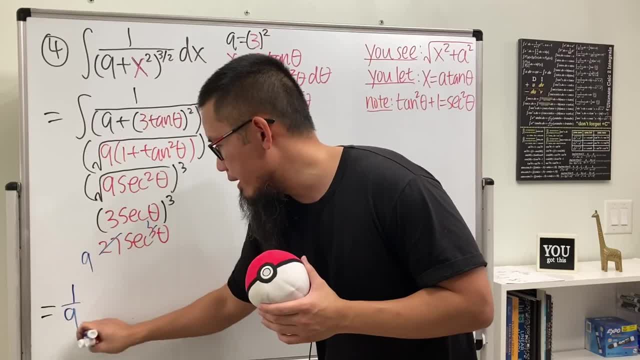 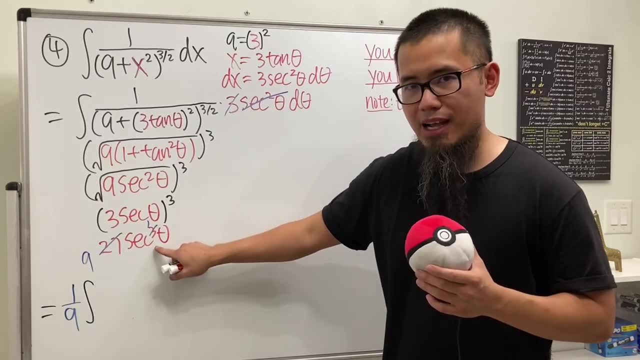 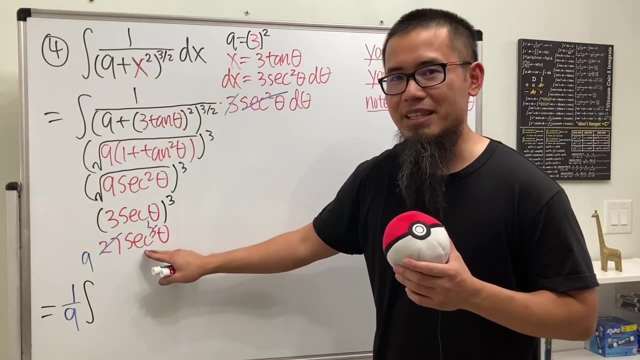 And let me just put that down all the way in the front of the integral. And then we have the integral 1 over secant, theta, Secant is 1 over cosine. 1 over secant is the same as just cosine. 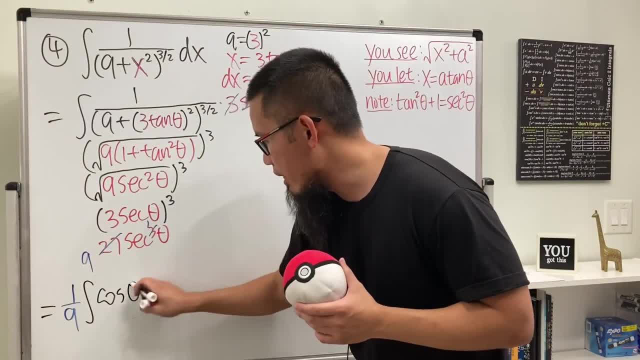 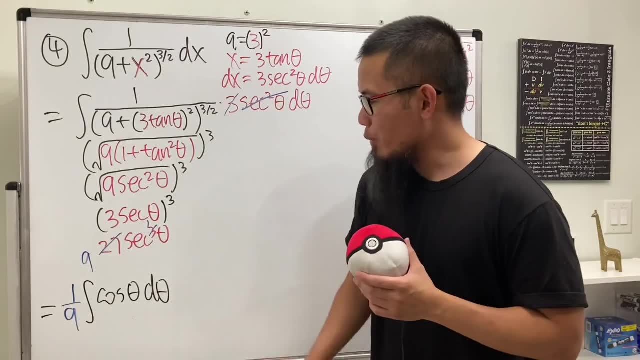 So the inside here is actually just cosine theta, Yep. So I told you this right here is actually easier than the other one. So that's what we have. Of course, to integrate this, we'll just do 1 over 9.. 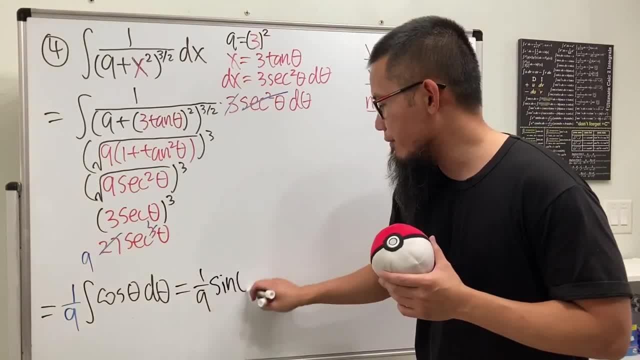 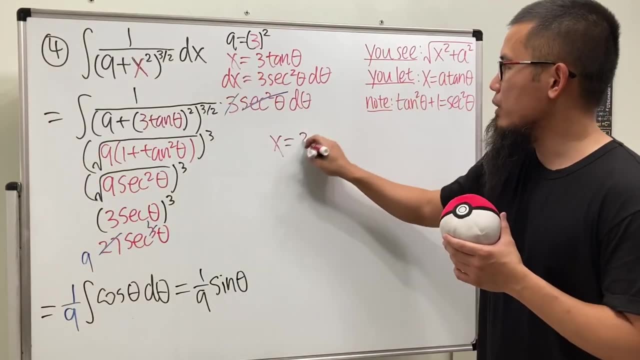 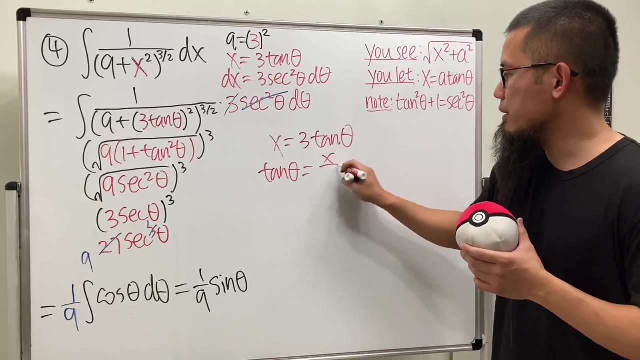 And the integral of cosine is positive sine. All right, And then at the end we just have to go back to the x-world. Take a look right here. We know x is equal to 3 times tangent theta. So that means tangent theta is equal to x over 3.. 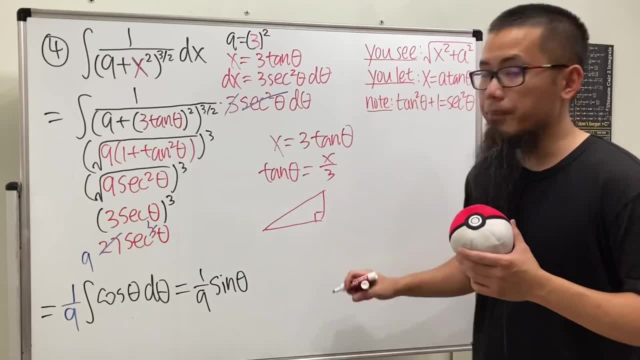 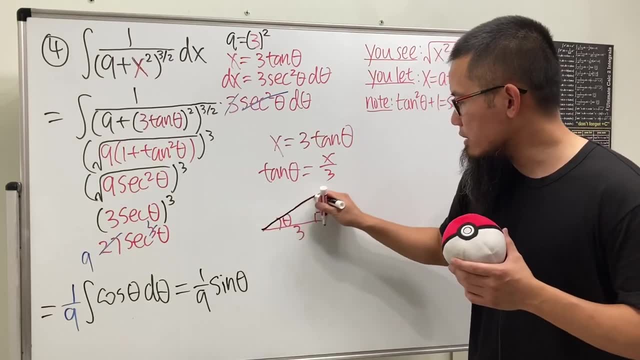 Draw a right triangle real quick. Right angle here, Angle theta here. This is the opposite. This is the adjacent And the hip-hop news is open, the square root, And we do this thing squared, Actually, yeah, this thing squared, because the 9 goes first.